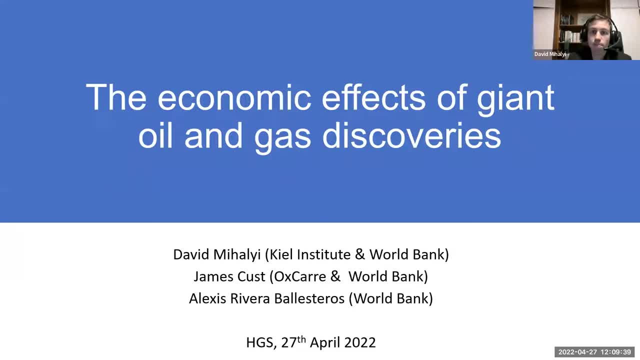 conversation to me. um, so this, uh, this is, as mentioned that, a paper that we did, uh for the aapg memoir. uh, and it's basically summarizing some of the research, the economic research, on the impact of oil and gas discoveries. uh, that's that's what we, uh, we wrote. uh, that's what 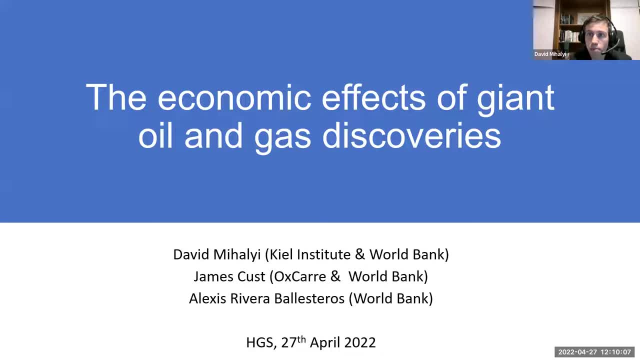 we wrote that chapter on and it's building on um, um on some of our own work but also other other scholars in in the field. so, um, i'm now uh this, this paper, and this research agenda is part of of uh my research that i do at the keel institute. 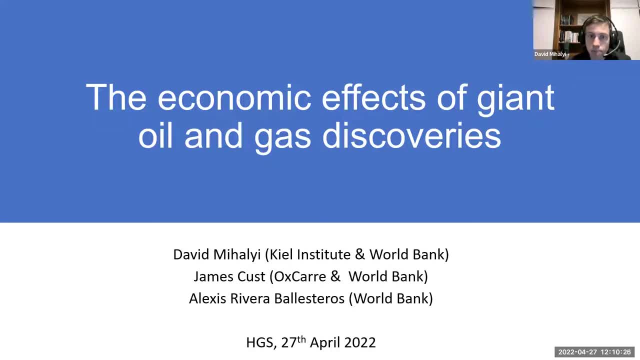 uh, where i'm a phd candidate but i'm also an economist at the world bank, but everything i say is not not world bank, uh opinion, or world bank affiliate, uh, doesn't represent the world bank's like that. uh, the the paper is actually co-authored with with the other colleagues also at the world. 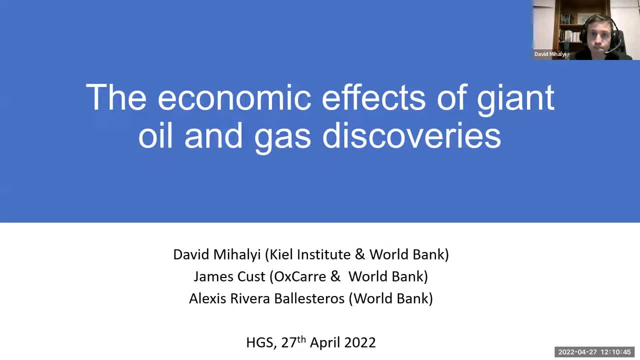 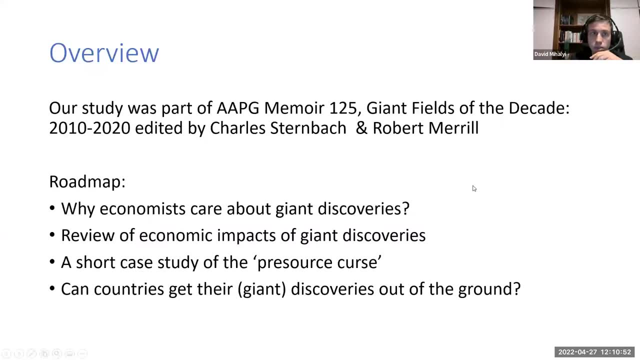 bank, james cust and alexis rivera balesteros. okay, with that, let me go to the next slide, if i can. okay, so, as i mentioned, this is, this is: uh, this study is part of of the aapg memoir, the latest one on giant discoveries, uh, and i'm gonna talk mainly about why we economists care about the. 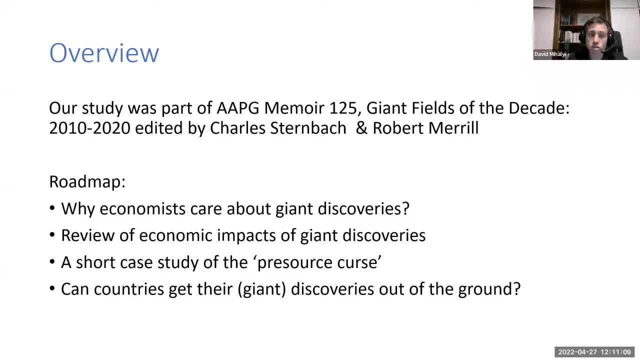 these discoveries. so i'm going to try to run through some of the key papers that discuss some of these economic impacts. then i'm going to give you a very, very brief preview of what we call uh with when uh with my co-authors. we call the pre-source girls uh, through a case study and then 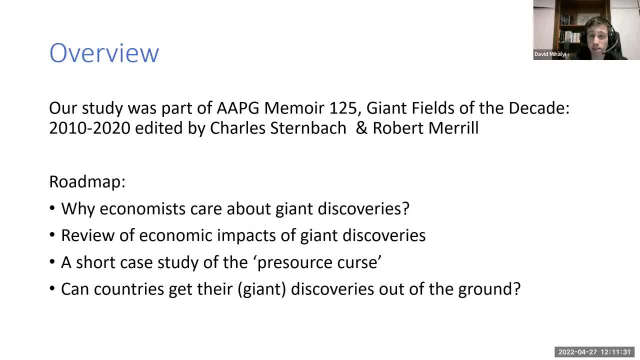 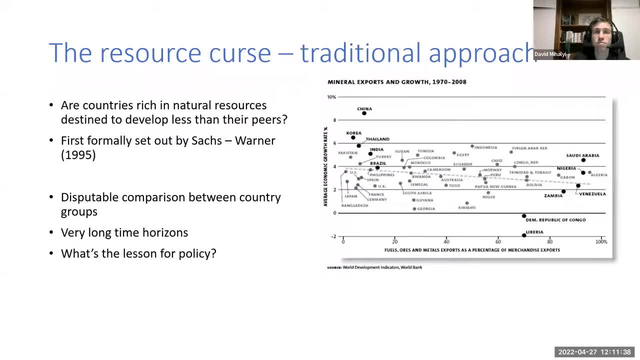 i'm going to talk about some, some of my latest work, which is about getting giant discoveries, or any discoveries, really out of the ground, uh, uh, okay. so the resource curse. i'm sure many of you you know this is economics textbook for us, but i'm sure, as geologists working on in the sector, you came across, uh, the phenomenon of the resource. 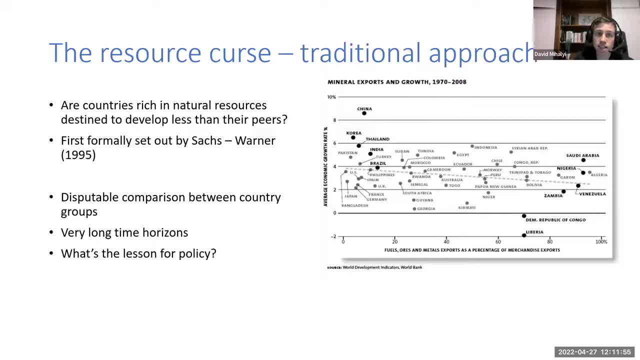 because this idea that countries that are rich in natural resources might be doomed to develop more slowly or or or stay poor. uh, this hypothesis has been around for a long time, for a long long time, going back to the idea that, you know, the spanish failed to industrialize. 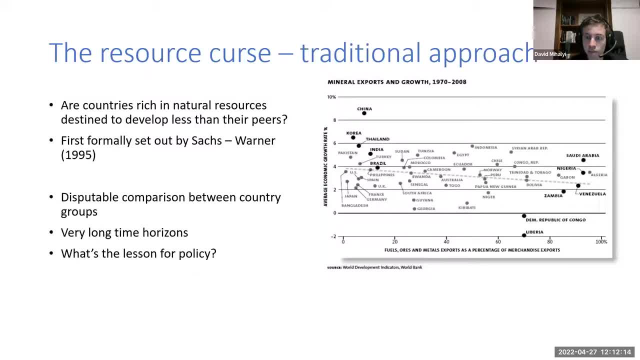 because all all the gold inflow that they had uh from, uh from the conquests, uh in the in the 15 and uh 1500s. but it was more formally set out by uh jeffrey sachs and michael warner in a paper in. 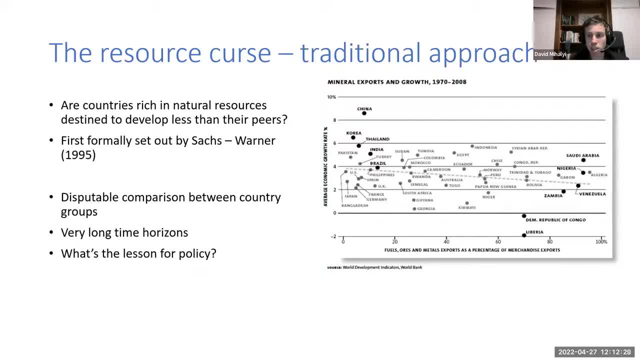 1995, which basically found this correlation, negative correlation, where countries that are rich in and very dependent on uh, few or in metals exports, so resource exports, that's on the on the x-axis on the graph, the countries that are most dependent, like nigeria, arabia, venezuela, zambia at the time this is, this was. 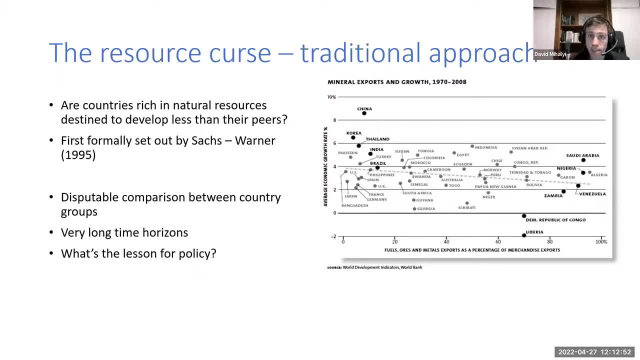 measured in 1970, are the countries that experience experience the lower level of growth than the countries that were not, uh, reliant on these primary exports, basically, so that was, that was this sort of sort of basic paper, uh, that we all learn in in textbooks. uh. this has since been, you know, disputed a lot. 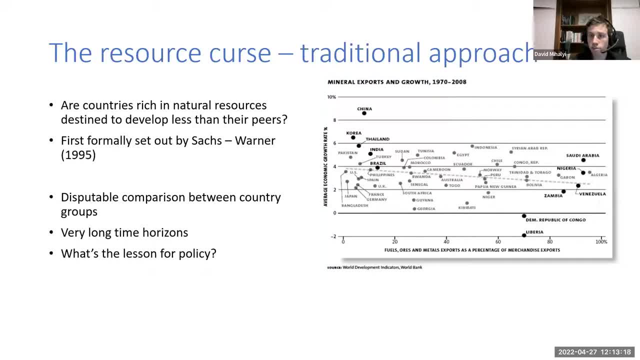 there's. it's a disputable comparison when you look at countries that you know, uh, that are very different, uh, rich and poor, geographically, all sorts. it's also very, very long time. horizons, right, this paper goes back to 1970. some papers go further, even further back, and we don't learn a ton. 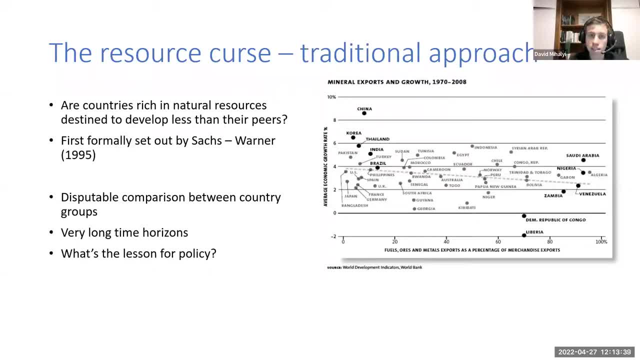 from, from comparing, from looking at these, these very long arcs, uh, across very different countries, especially in terms of the policy lessons. yes, don't don't be nigeria, but what does it mean? don't be nigeria, uh, or don't be congo? is there, is there anything actionable in terms of what? what is it? 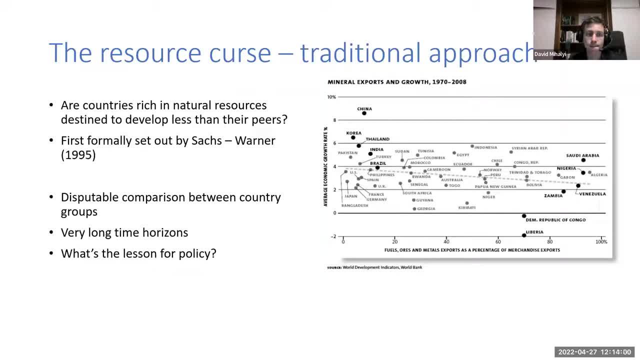 one country doing right or one country doing wrong. uh and, and you know, over 30, 40 year horizons is very, very hard to discern uh, patterns, obvious patterns of policy. Obviously you can make assertions around culture and sort of deeper things, But in terms of policy choices that these countries made, it's very hard to. 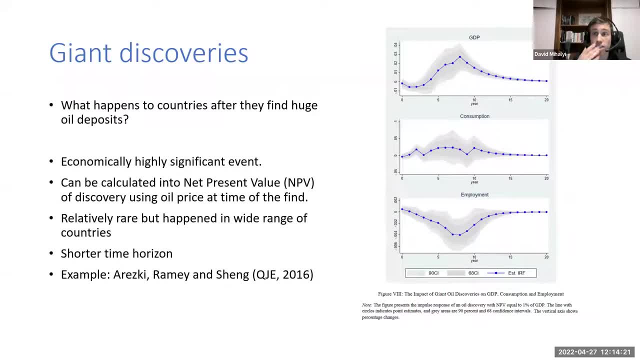 capture any of that in that kind of time horizon. There's a new strand of research and that's what got us excited. That's not trying to compare resource-rich and resource-poor countries. Rather, it's looking at countries immediately or soon after they make a big discovery. So you can 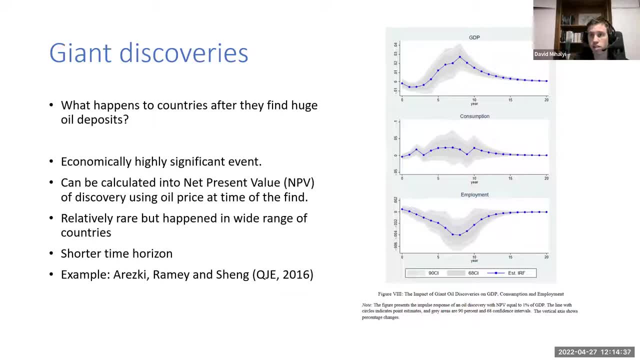 look at the country before the discovery or after the discovery, You can look at countries that are very similar just around the same years. Economists think of it as a cleaner comparison, to use what they sometimes call difference in difference, where you look at the trends. 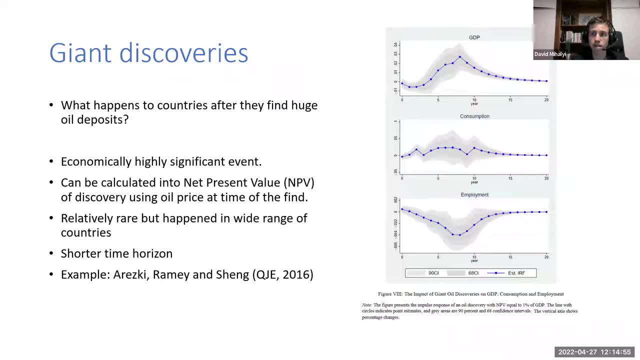 of a bunch of countries and one of them makes a discovery, say, in a particular year, And then you can sort of keep continuing to compare for a couple of years whether the trend of the country that made a discovery It differs from its peer group, basically. So what happens to these countries after they find these? 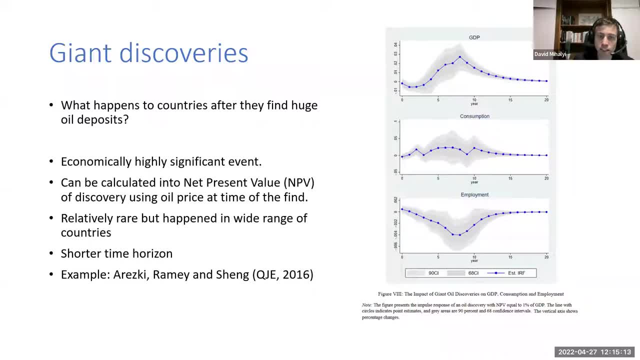 huge oil deposits. The first big paper of this type is quite recent. It was published in the Quarterly Journal of Economics, which is the most prestigious journal of our field, by Rabar Eski and co-authors, And it finds that these are that you can basically very clearly see the impact of 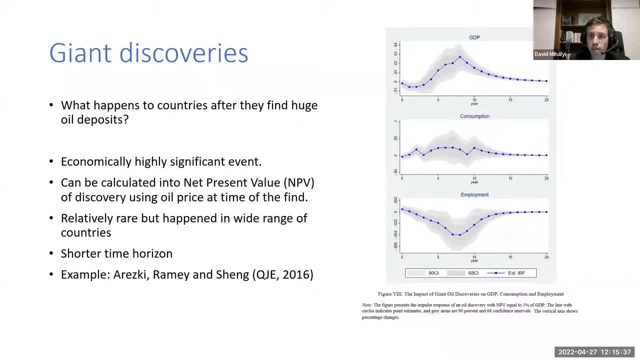 discoveries. in the macroeconomy, in the economic data, You see GDP jumps five years after the discovery is found. That's what you see on the right side. You see consumption doesn't move that much and you see a negative effect on employment after the discovery. And then they do a lot more. 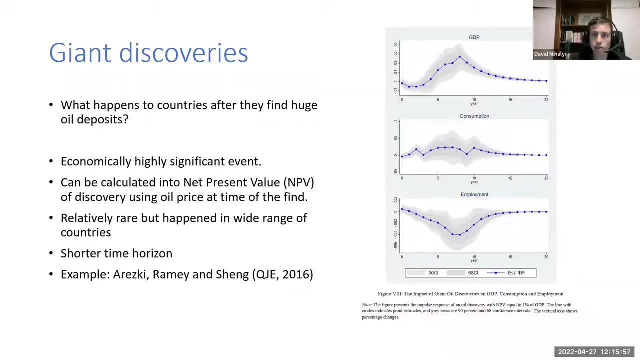 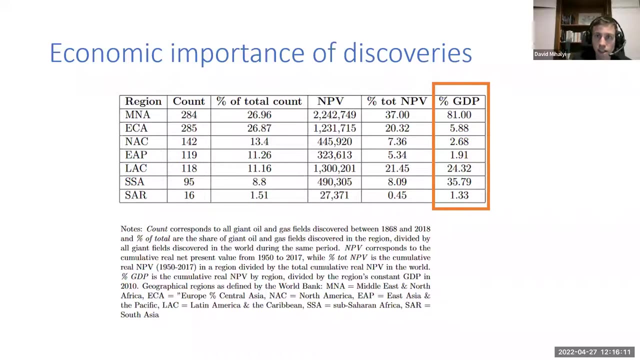 of these kind of analyses. I'm just showing you as an example of how you can use exactly the moment, the timing of this discovery, And look at how it impacts these macroeconomic variables. I'm going to give you more examples of this sort in a minute. But the big question is: how do we so? how do we use this discovery data? 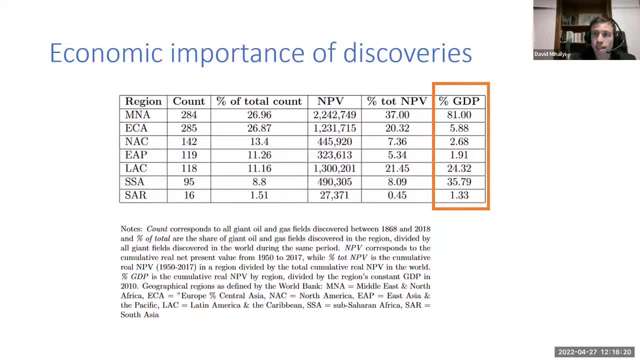 Well, the main way we use this discovery data is we just don't just look at the event itself, We also look at the size of the event. And to calculate the size of the event we do what's called what we call net present value calculations, where we take the 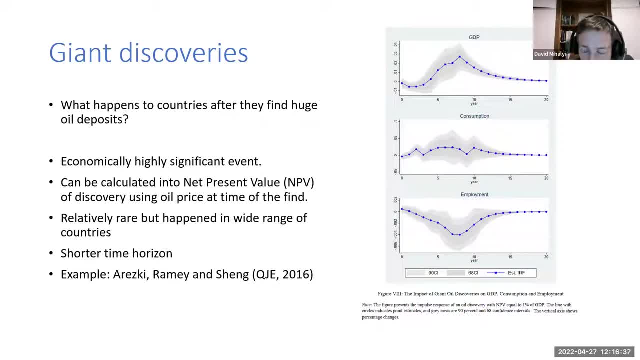 well, we take the estimate, estimated ultimately recoverable reserves- which I know is a debatable concept and all that- but we take whatever numbers we found in the giant discovery data sets in terms of recoverable reserves, recoverable resources. Sorry, I'm getting confused already- And URR. 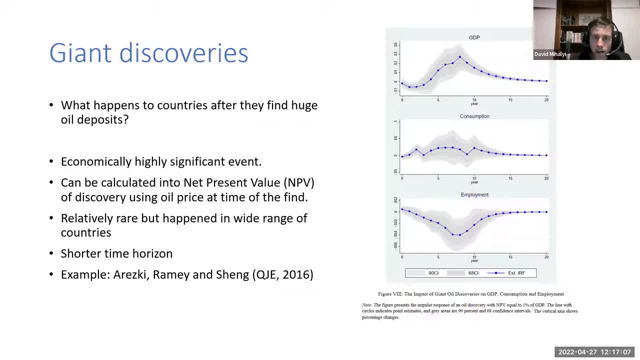 And, and then take the price at the moment of the discovery and then do a calculation in terms of you know, maybe it takes 30 years, or we take sort of an average curve. Well, this is what the Aresky paper did. It take the average curve in terms of how many years it might take to extract that oil. 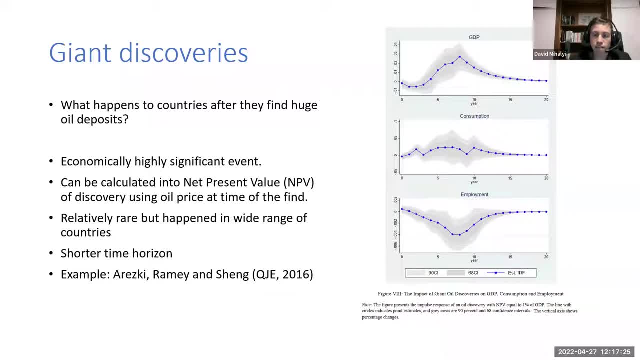 and sort of calculates the value, the value of that flow, the value of that money flow. Obviously, it's going to be very imprecise, but the idea is: is that a discovery? you know, 500 million barrels is different for Guyana than it is for the United States. 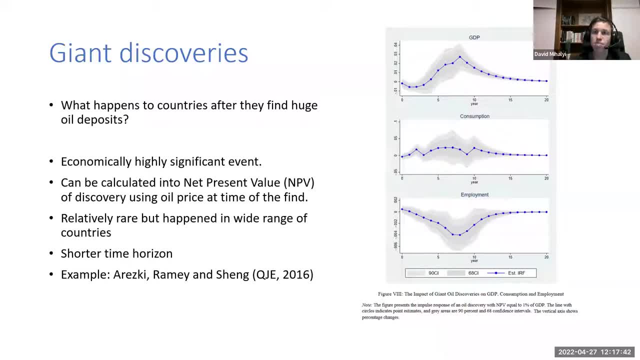 right, And to get those numbers into perspective, we calculate it as a percentage GDP, which is, again, is an imprecise measure of the size of the economy of the country, But it gets to the idea that, you know, this same giant discovery might mean very different thing for one country than 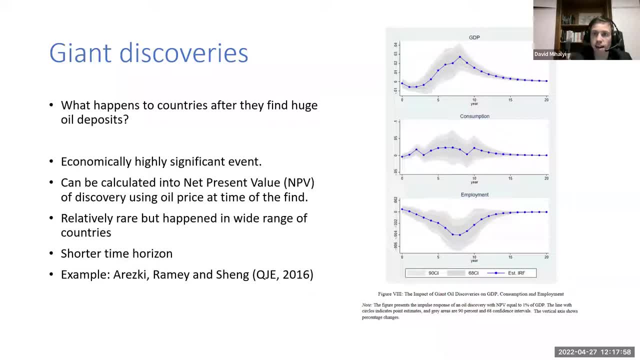 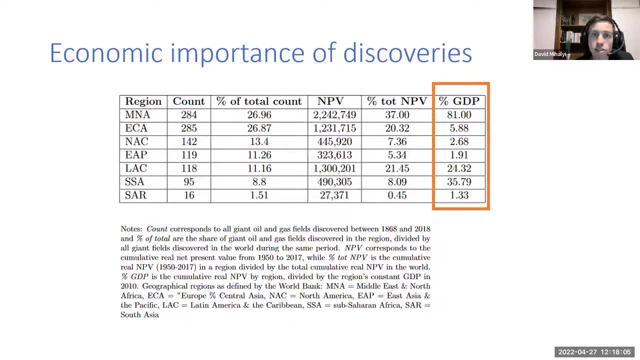 another country And it puts basically a dollar value and then a percentage GDP value to that discovery. And so we did that You can. we looked at the. we did it across regions And one interesting thing you see in the data is that if you just 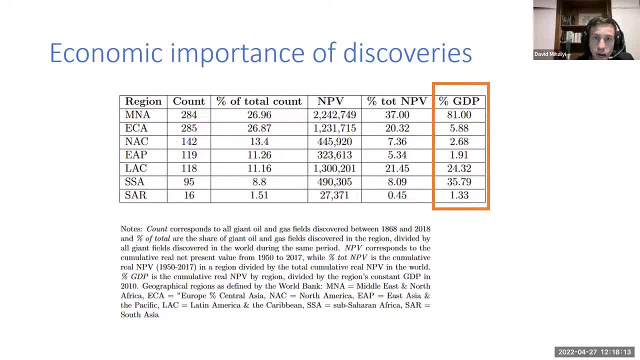 look at the, the, the, the count of discoveries and where they happen. we see that a quarter of them happens in the, in the Middle East and and North Africa region, for example. We see that in terms of their total value, as in the, in their, their total value, yeah. 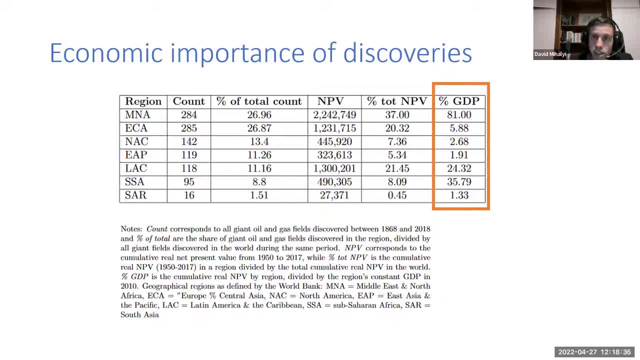 is is the largest again in the Middle Eastern region, And then you see their values as as well as percentage GDP, And again Middle East will come out first. but you also see that, for example, South Sub-Saharan Africa, SSA- it has a relatively low count of discoveries. 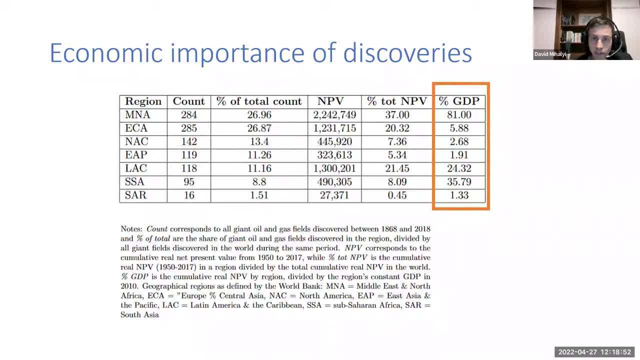 and a relatively low value in terms of of of the value of the discoveries in in billion dollars, But as percentage GDP it's it's rather significant: 35% of the continent's GDP, based on this estimate, is found in this in terms of discoveries. 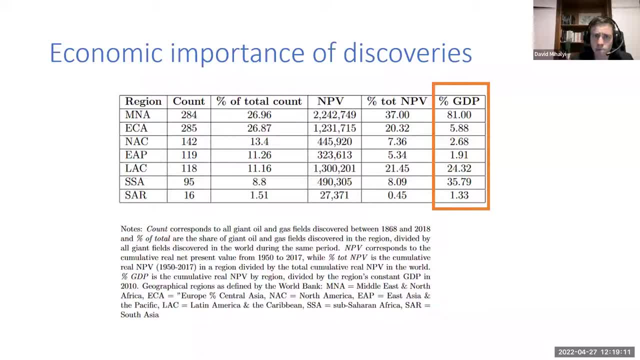 throughout the 1950 to 2017 period. that for period. that's the period we we've been using, because GDP data is very unreliable in for 1950, basically, and the countries were not the same in many cases. So this is, this is discoveries by decades. 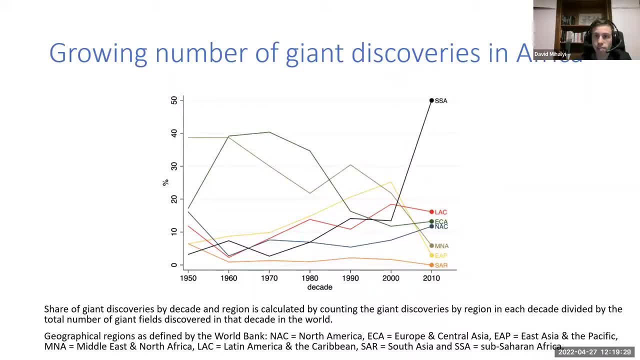 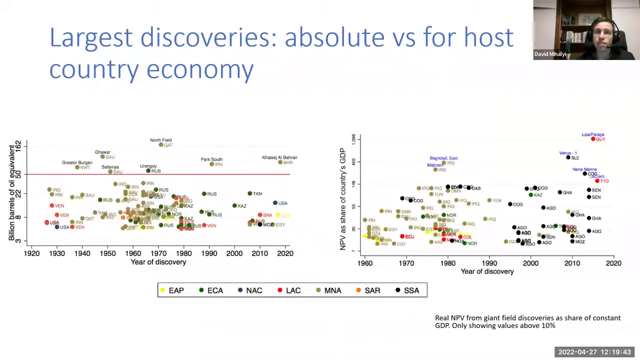 and there you see that actually Sub-Saharan Africa and Latin America are are actually increasing in trends in terms of the number of discoveries- We just mentioned Guyana making record numbers of giant discoveries- and in terms of size as well. But even more interesting for us is not the 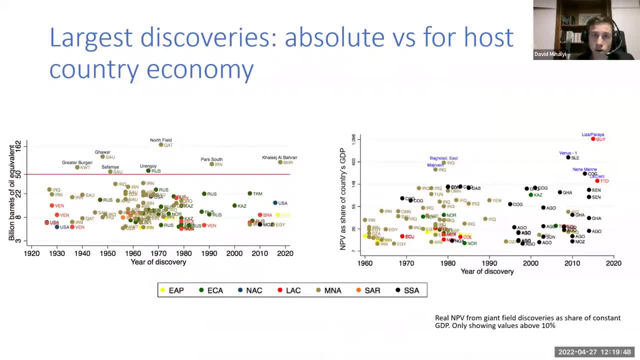 absolute number of discoveries, as I said, but the value for the host economy. So in terms of billions of barrels, again you see Kuwait. Russia saw these on the left side as the big discoveries. This is, it's not a linear scale, it's a log scale, but again you see these hundred. 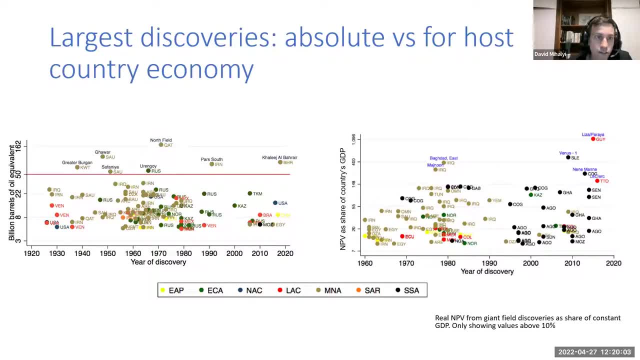 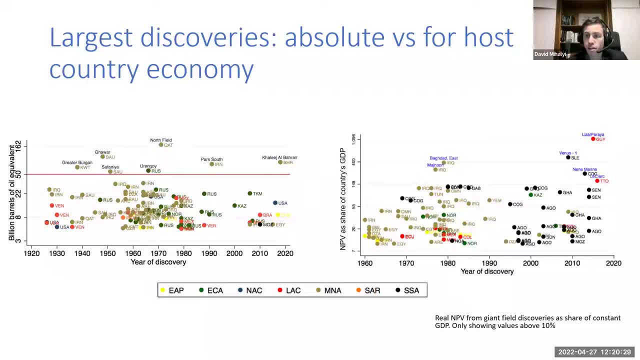 share of the share of the country's economy. And then you get very different countries that are sort of that made very big discoveries. So, for example, you see the Guyana one we just mentioned. this is the first LISA discovery that we have there, because the latest ones weren't included. 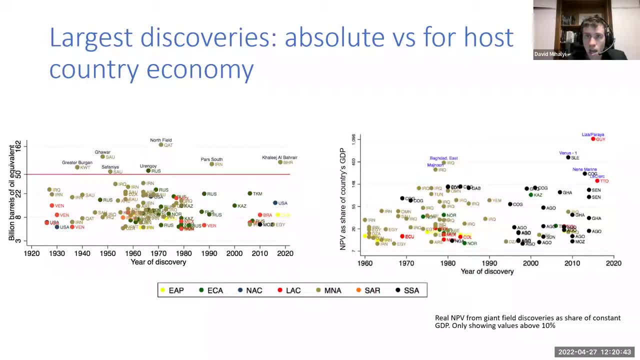 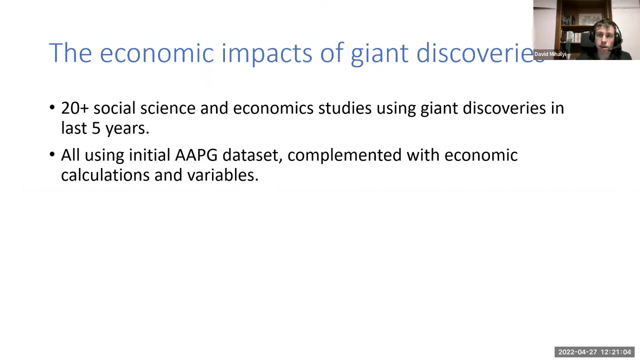 in the data set. yet And then. but you also see the Sierra Leone, Venus, one discovery- Congo, Trinidad- have made very, very significant, very significant discoveries in terms of countries' own GDP. So we have these measures right. For us, this is what matters the most. We have these. 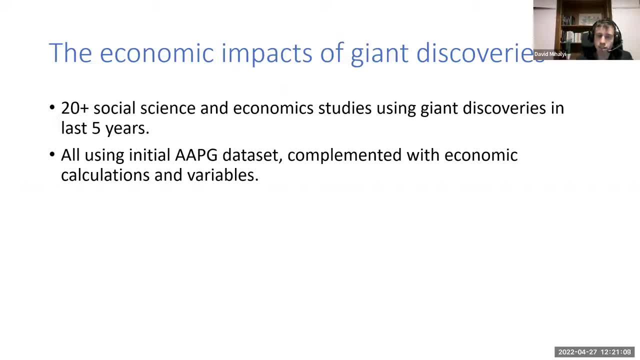 measures of discoveries in terms of the size, as measured in the size of the country's economy in net present value terms, And that type of measure has been applied and used in over 20 social science papers that all use this. Let's look at where where there have been 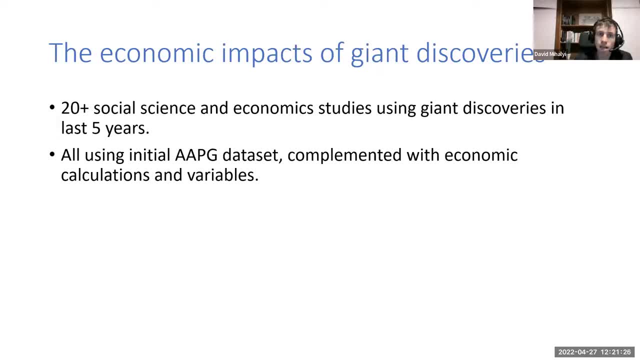 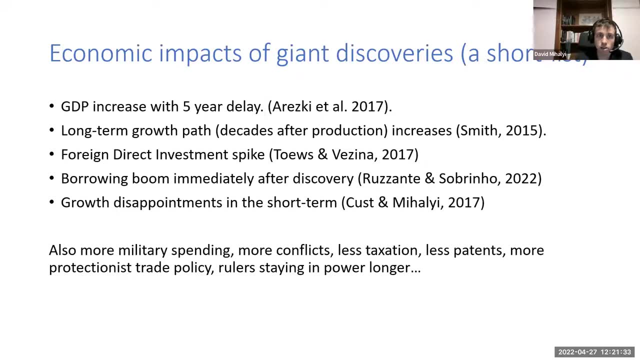 the biggest discovery shocks for the economy? What impact did it have on various social indicators And these 20 papers? I mentioned the Aresky et al QG paper from 2017, which was looking at, which found which was the first big 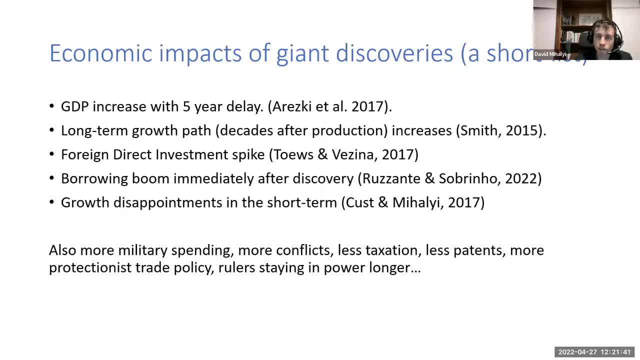 one and saw these big jumps in GDP five year after discovery, but also investment growth and but also declines in employment. But then we saw there was there was actually an earlier paper that made less waves. that was looking at long-term patterns, decades after production. 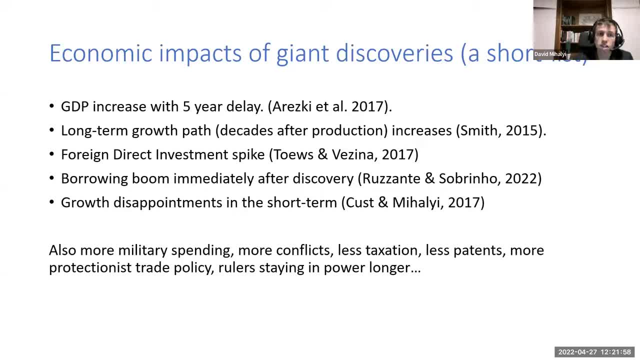 To be fair. But then there's other papers that look at investment spike in other sectors, by Toevs and Bezina. There's a paper by Rizante and Sobrino that's focused on on the borrowing boom that happens immediately after discovery, which is quite similar to our own paper, which 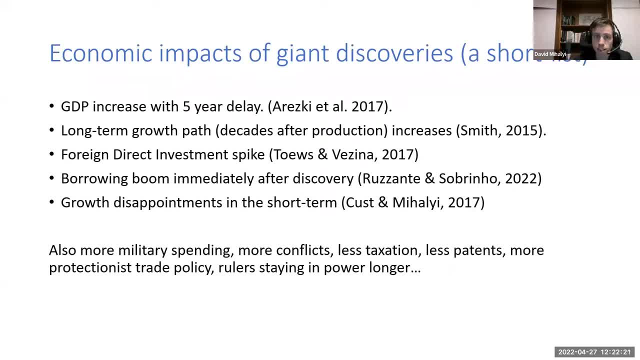 I'm going to talk a little bit about, which looks at the short-term impacts of these discoveries- Some other papers that are out there just to mention briefly. giant discoveries are associated with an increase in military spending or conflicts. less taxation, less patents, So less innovation. basically more. 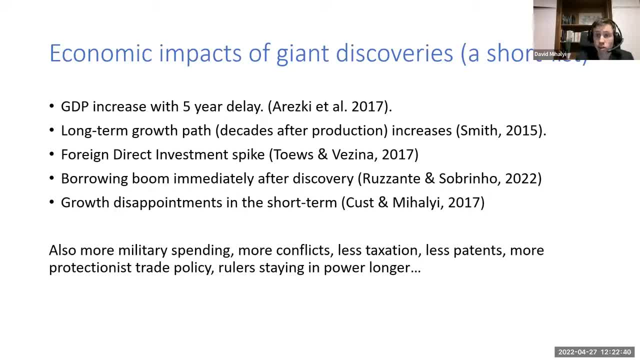 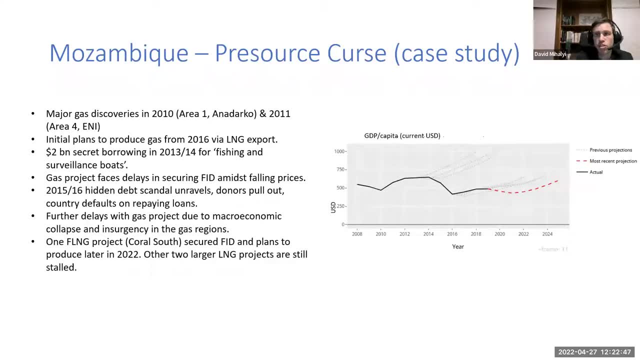 protectionist trade policies, rulers staying in power for longer if if they happen to have a discovery while they're in power. So the pre-source curse hypothesis that we put forward with with my co-author, was the idea: the countries, some countries, 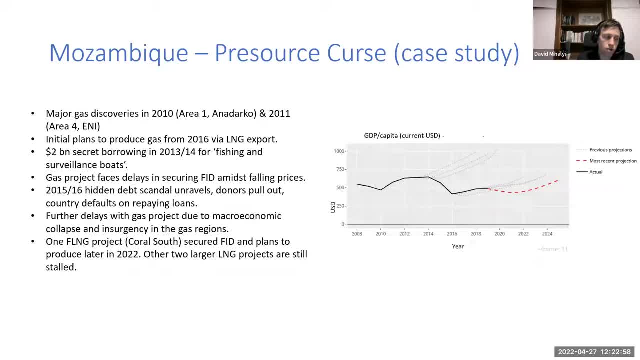 in in countries with, and we were focused on on what we call countries with weak institutions. So these are often countries that that sort of the lowest level of human capital and the less relied and then the worst performance on various metrics of, of of rule of law and 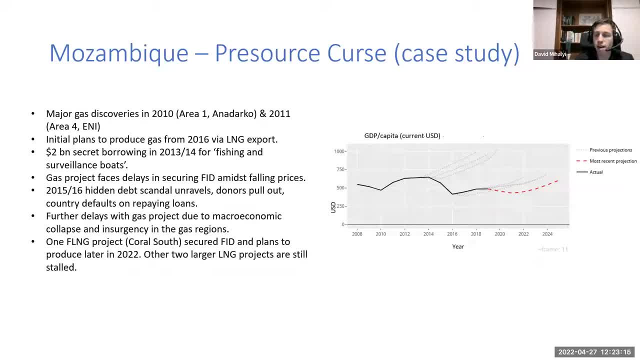 and other measures of that nature. They, what we found is: soon after giant discoveries: they have. they have a big short. there's there's a there's a big optimism in terms of their expected growth trajectory. They, what we found is: soon after giant discoveries: they have. they have a big short. there's there's a there's a big optimism in terms of their expected growth trajectory. 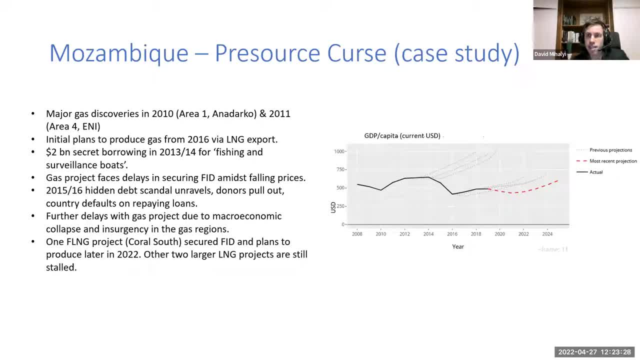 as measured by IMF forecasts, And what we found is that these countries signify always well, systematically fall short of the expected boom that that you know the IMF was projecting in these countries, And one case study of that is is the Mozambique discoveries in 2010 and 2011,, where the 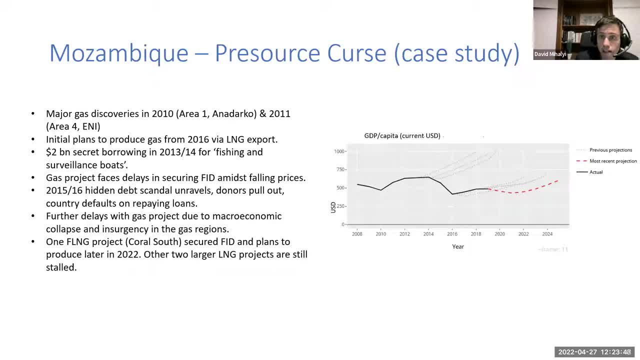 initial plan was to produce gas from 2016, mainly via well, by LNG export, mainly onshore. And then, two years after, there was a big scandal where the government borrowed in secret. This was not authorized by parliament. They provided state guarantees to to a state-owned company to 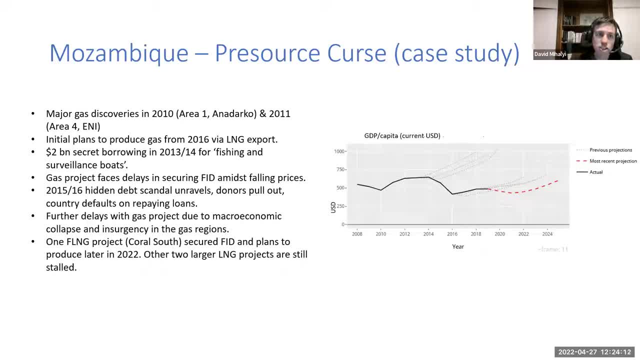 purchase to buy what was, you know, deemed fishing and surveillance boats $2 billion. There's now court cases and and, and actually even verdicts Against the banks that were involved and then the borrowers that were involved, Anyways. so that's, that's on the corruption side of things, but also it meant that the but there. 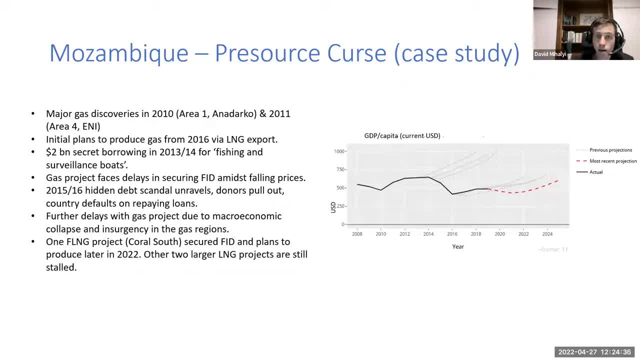 was also the fact that the gas projects basically were delayed, not I mean partly because of the falling gas prices, but also because how the hidden debt scandal unraveled, which meant that donors pulled out the country defaulted on on on on repaying its own loans. 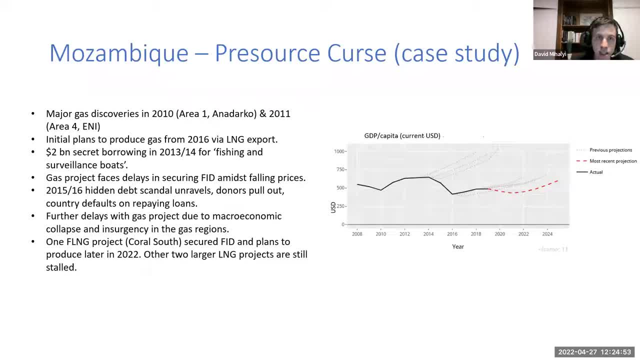 And so these macroeconomic problems created further uncertainty As well, as there was insert, and now- well, a bit later, there was also insurgency in the gas regions. So basically, only one, the smallest one, the FLNG is is- has secured FID. the other, the bigger, 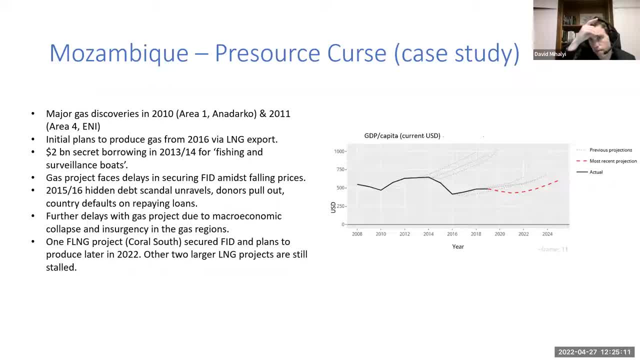 projects are, are still stalled, And and the Mozambique story is, you know, Mozambique was, was actually, you know, projected to grow very, very rapidly and on the back of the growth, on the back of these, these gas discoveries. 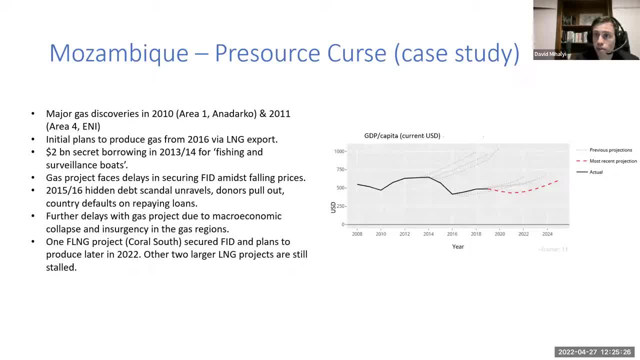 And to date, obviously, the country has become poorer in in nominal terms than than it was before it found the gas. So that's the kind of problem that that we we highlight and analyze more systematically in our paper on the pre-source curse. We like to call it the pre-source curse. 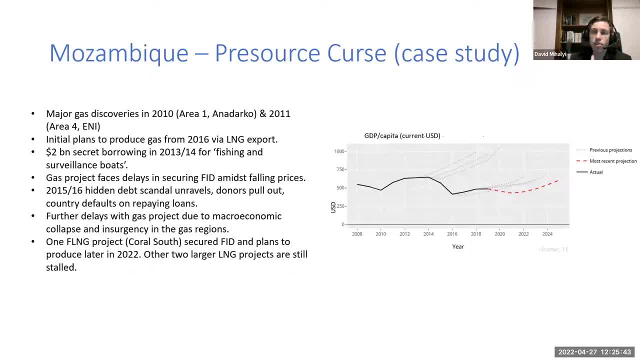 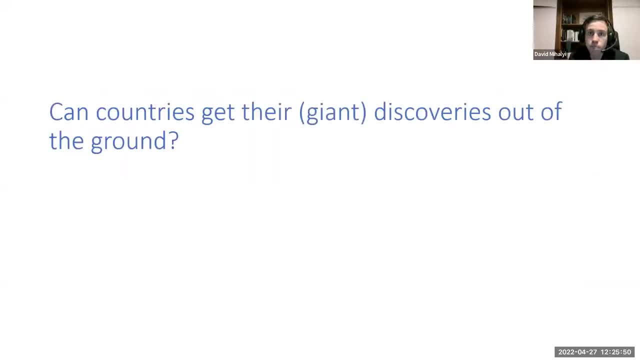 because it happens before the actual resource curse comes in, right At the moment of discovery and way before you become really dependent on the oil and gas revenues. That's the idea. So another problem that I'm focusing in my new research right now, which is still in a very 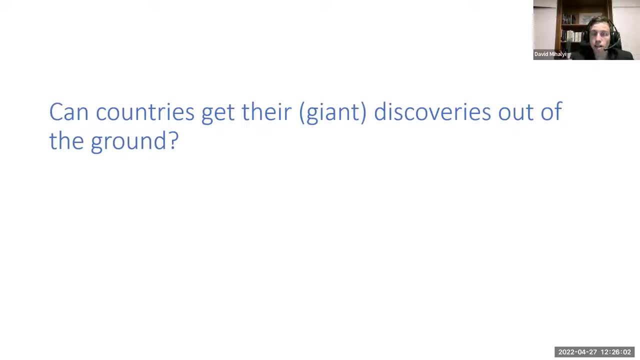 draft form we have working paper on- well, I have a working paper out- is whether is what take, what it takes for countries to get discoveries out of the ground. Obviously, the Mozambique case is also one of those where a big part of the problem is the country still not producing the gas. 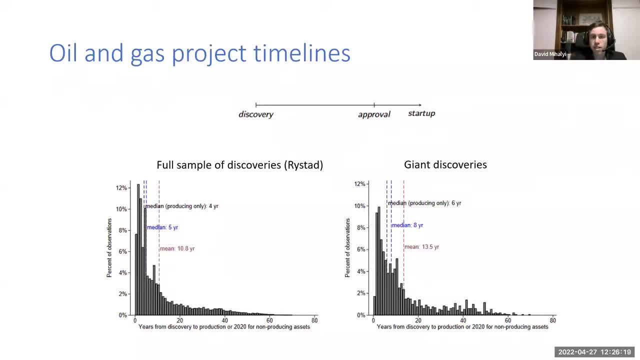 And it didn't even reach final investment decision on the on the bigger projects. So I studied Christian Brog対 is also one of those where a big part of the problem is between discovery to approval stage to startup stage. i've used both the giant discoveries data. 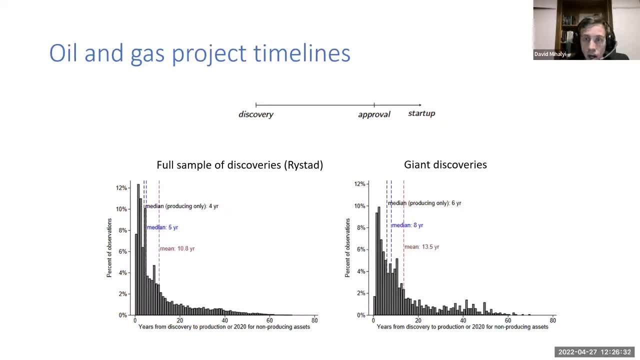 set initially by aapg, uh and uh, and a full sample of discoveries by rice stats uq platform, and i can see, for all of these discoveries- uh, actually, i'm sorry this is for this- is this whole analysis is based on, on the rice, that data, because that's the one that gives me approval. 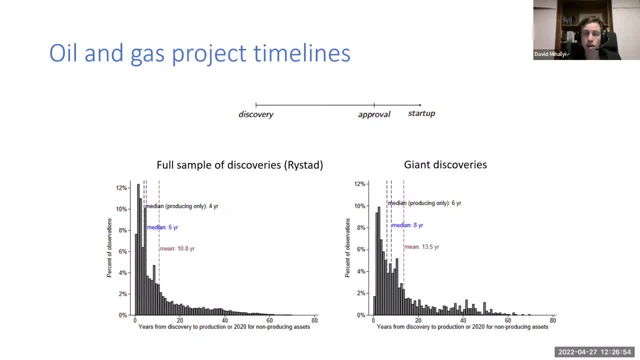 dates and start updates on a standardized form, but i'm looking at both all discoveries and discoveries that are beyond 500 million barrels, uh, and what i see in the data is most discoveries that reach production. they come online within four years. or for the giant discovery, it takes about six years to for for the ones that came online to come online. but there's 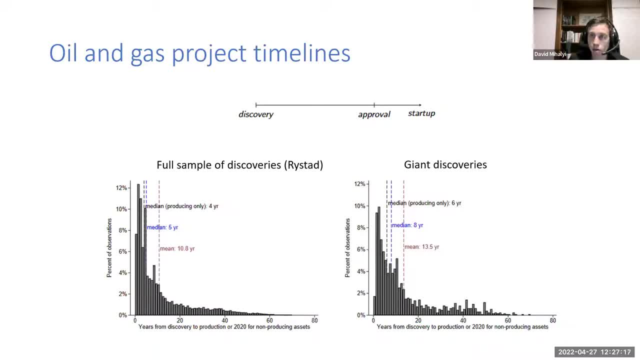 a long tail of discoveries that never reach production or or that take a long, long time. so most discoveries, again, as i said, very relatively rapid, so close to the five years that- uh, that was actually put forward in the in the risky paper- is the average time it takes to get giant discoveries. 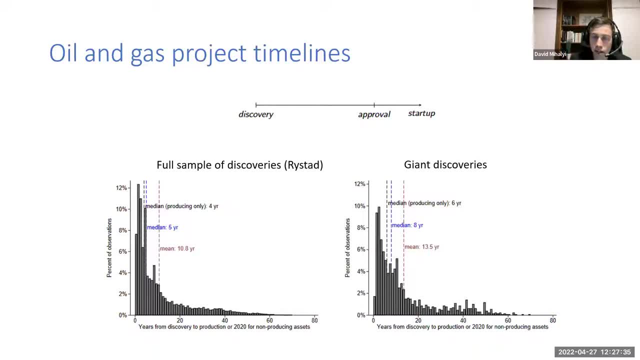 out of the ground. but actually, you know, if you include all the discoveries that never got to production, then that are, that median value is actually more like for giants, more like 80 years, and if you, uh, if you include all the discoveries that are still not producing with a 20, 20 year, 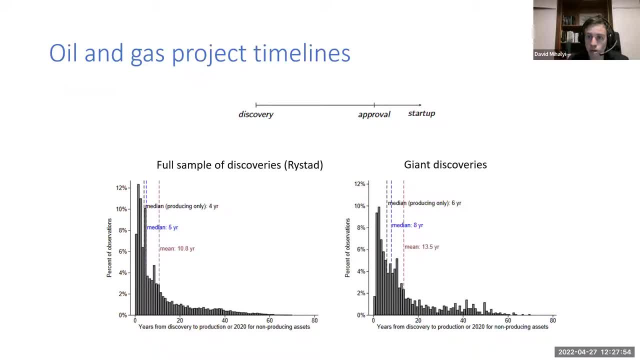 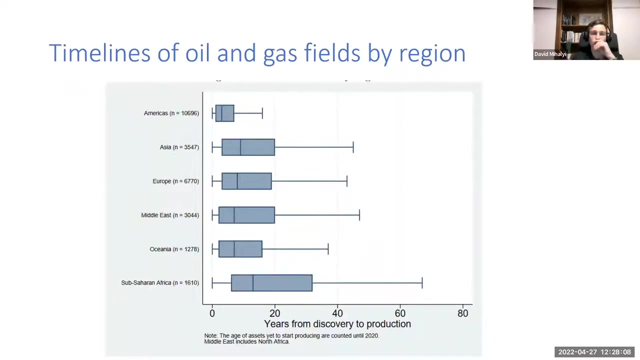 you get these, you get these discoveries that have been underground for 40, 50, 60 years in in some instances. i mean, obviously these are more. these are relatively rare, but it's not uncommon to have 10, 20 years in the ground, and so i looked at the split by region and then i do more statistical analysis where i control for 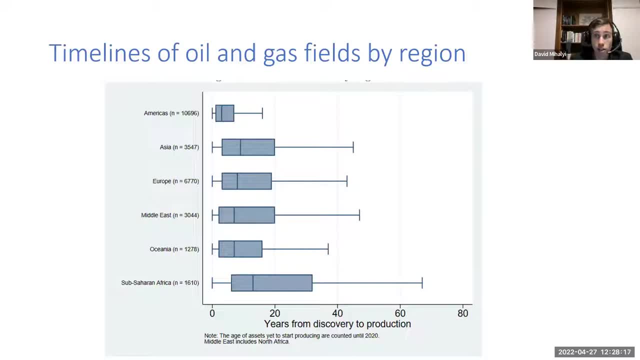 the size of the discovery, whether it's onshore or offshore, whether it's oil or gas, whether it's how deep it is, and, i add, all the various controls and the patterns stay relatively similar. i don't want to dump very complicated statistical models into into this discussion, but i'm uh, but i do want to. 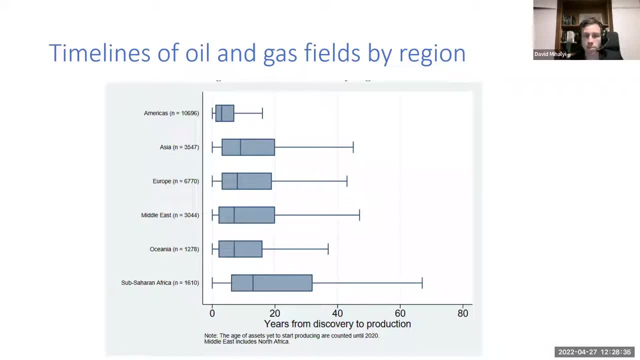 sort of highlight. the key takeaway, which again is very obvious in the patents, is these countries with weaker institutional scores, many of them in sub-saharan africa, have these very, very long timelines. so you know, in north america especially it's very uh, not just the shale, but of course i'm 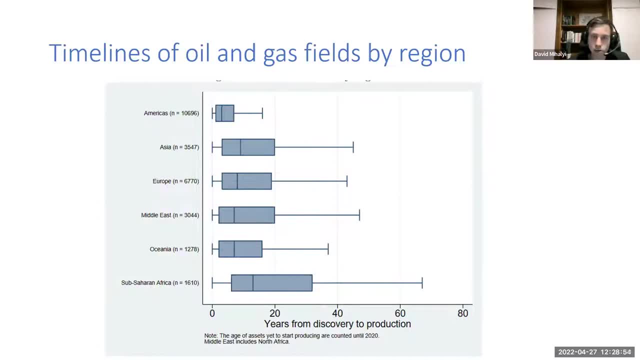 also the, the the sort of regular or it's very quick to get out of the ground. uh, i've actually excluded shale from a lot of the analysis. uh, whereas, as i said, sub-saharan africa, but not only sub-saharan africa, not wanting to single them out- a lot of countries with weaker institutional 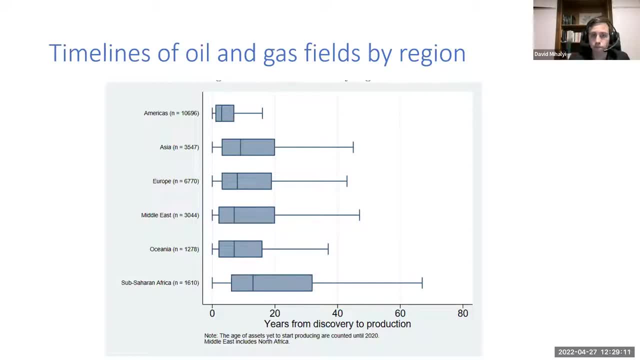 capacities. they have these very long timelines often or, if you will put it another way, very struggle to get final investment decision on the discoveries. and if they do, even it takes longer to get from the decision to uh to to actual production, both for oil and especially for gas. 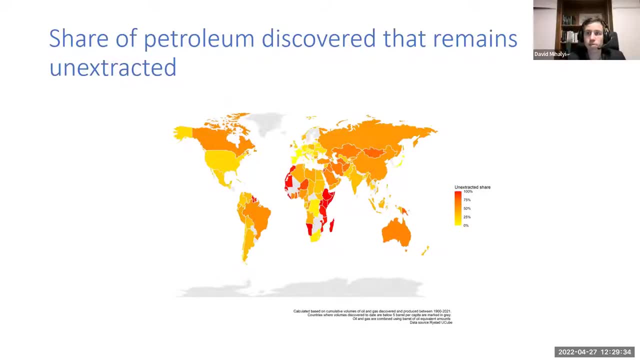 okay, and then this is the final, the sort of thought-provoking- i hope so provoking- graph that i did, which looks at the total value of resources discovered. again, this is not so, this is not proven reserves, this is resources discovered and i've, uh, and i've divided well, so 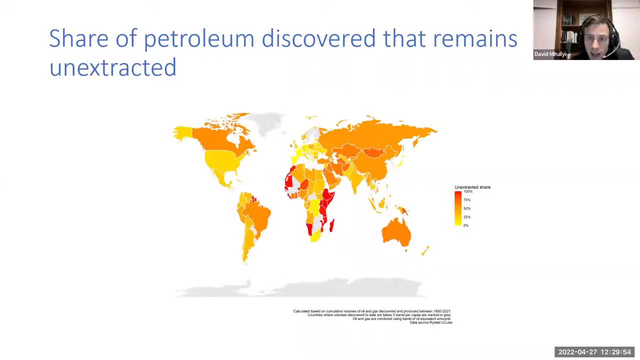 look at the total production, uh, as a share of of what was found, and what i see is that countries, richer countries uh, countries uh in in the west, uh, western europe, and then also the us- have extracted a relatively large share of what they found in in the past, since 1900. uh, that's how far. 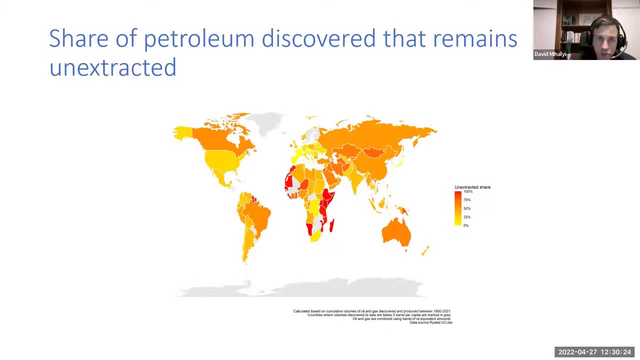 again, uh, uh, africa, but also guyana there, uh, obviously, uh, those are very recent discoveries, but the african ones are, are, you know, some of them are 10, 10 years old discoveries. uh, they've they barely. many of these countries have not even started the extraction process. tanzania's gas. 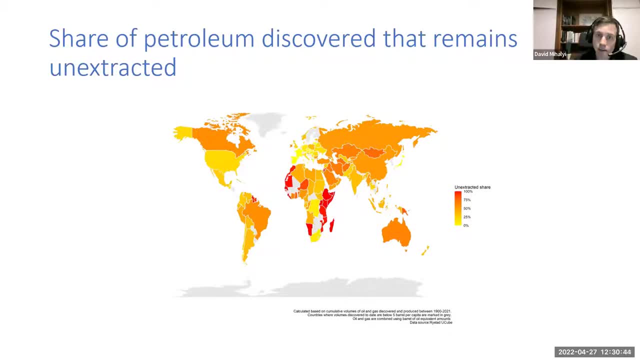 you can think of, uh, mauritania and senegal only only reaching final investment decision recently. so i think i'm interested in by this research because there's, i mean again we can debate how quickly energy transition might happen. but if there's an impetus for energy transition, meaning that- and i 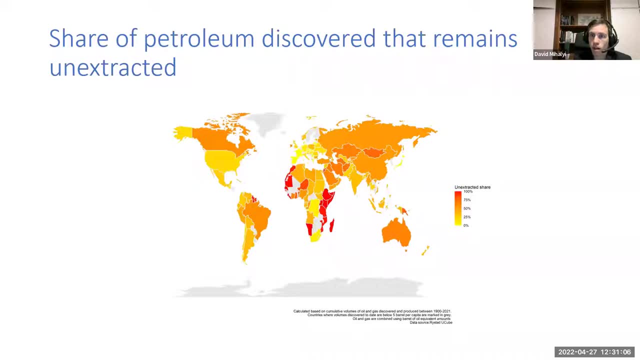 think it's clear that we are finding a lot more oil. there's a lot more oil being discovered and how much oil is being used up. so you know the there's there's more additional resources found than there is uh and if, if there is an acceleration towards more uh, less reliance on on on oil, then the 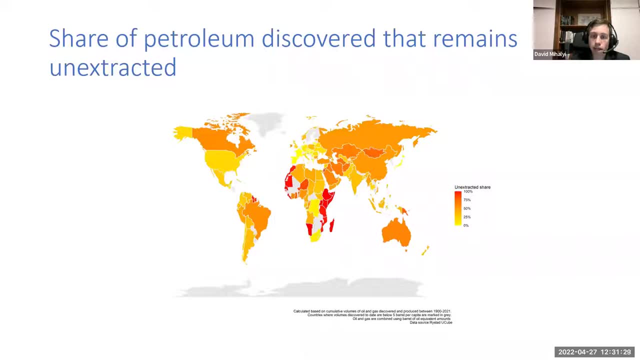 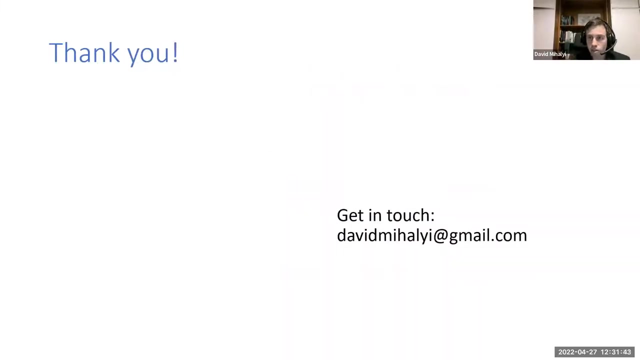 question is: will some of these countries be able to get it out of the ground, or will it? will it be stuck and then sort of stranded on the ground? so that's, that's, that's one way i think about this research on timeline. um, i'll stop here. thank you very much. uh, this, so this. this was what i prepared. 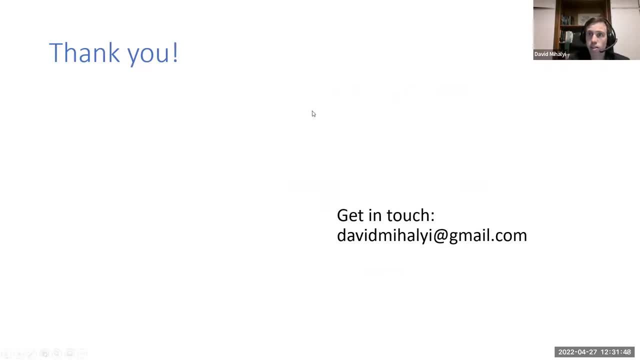 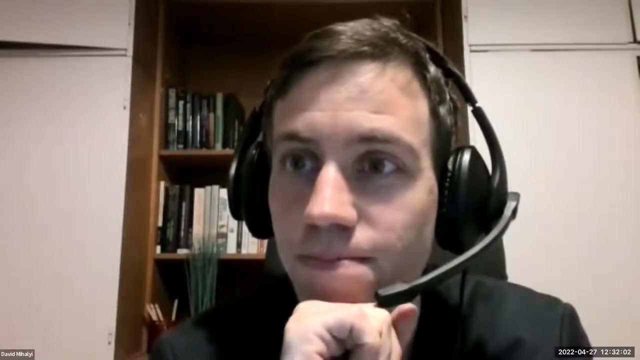 and i'm happy to answer questions and but also more, even more excited to hear some feedback on how it looks like, sounds, from a geologist perspective. david, thank you, i'll get you to stop sharing your screen, thank you, and i don't have any questions in the q a right now, but i got all kinds of questions in. 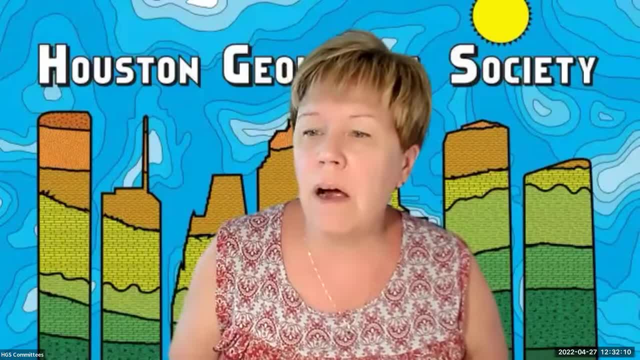 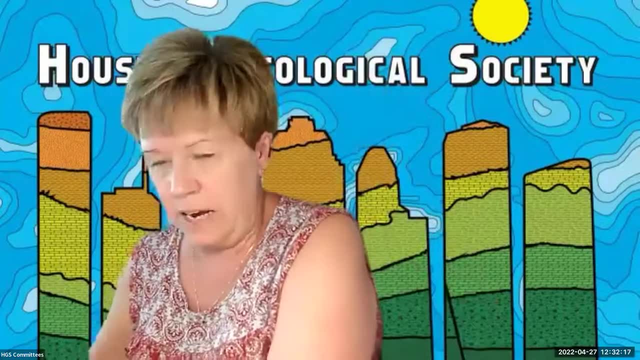 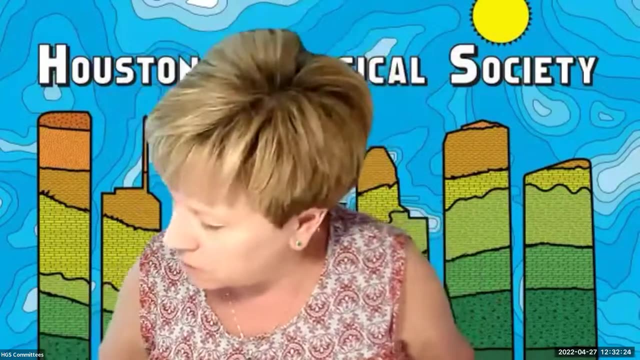 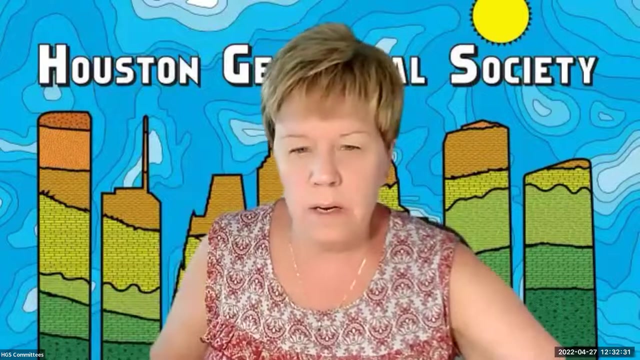 my head, um, and since we're a smaller crowd, if people can also just raise their hand or type a question in the chat- if you have one for david, um, this is fascinating to me. so so one question that i didn't understand: on your graph, why the negative effect? unemployment, i mean, it seems like when you look at what a lot. 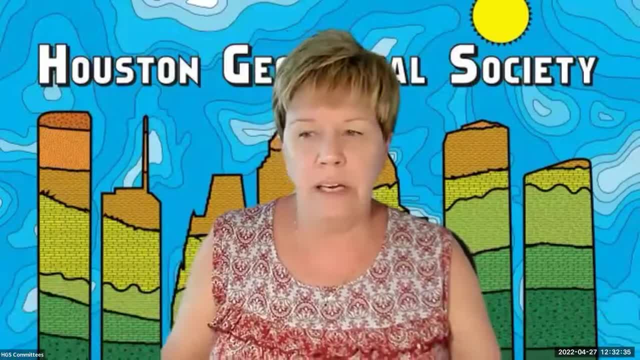 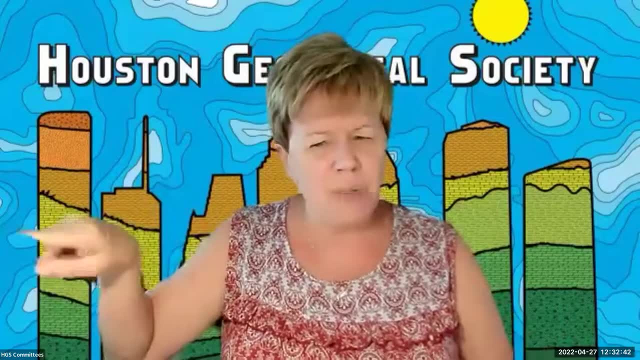 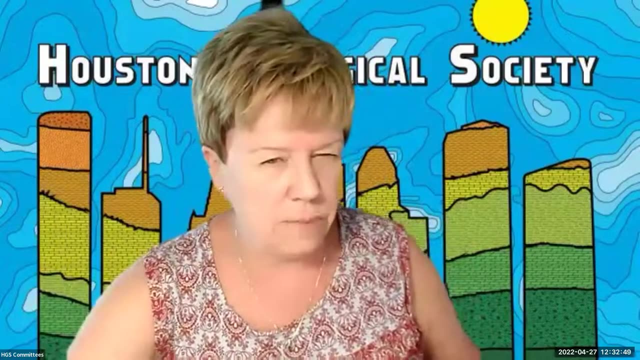 of companies go in and tout about making a major discovery in an area it's. it's the jobs it will bring, it's all of that. but your chart actually actually said something else, which i found very surprising: that there was a negative corollary with with employment. what do you think drives that? i think that's, uh, that's, it's evidence of something economists like to call the dutch disease, which is the idea that, uh, when you find oil, or when you start producing, especially, you get all of the dollar. dollar inflows into the country and that makes your currency appreciate. which means that's your economy, your other sectors become less competitive because you got such amount of dollar inflow. suddenly your currency becomes, uh, stronger, which means that if you're, say, a garment producer or whatnot, you you're facing cheaper, it's going to be much cheaper to import things. 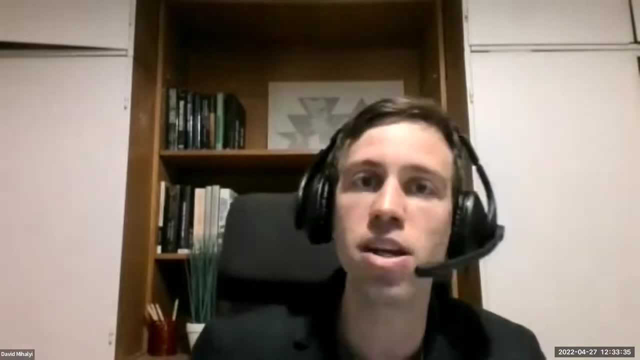 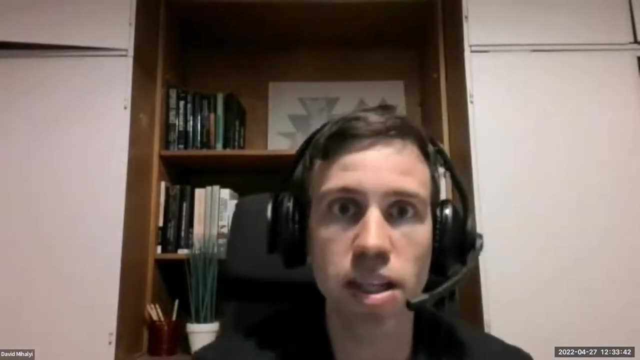 because everyone has dollars basically, and it's going to be a lot harder to be to remain competitive for an exporter of whatever rice or whatever else. so that could be. so that's that's one risk with the oil production. that's one of the ideas that's been put forward, that the reason oil, oil. rich countries are struggling in all their other sectors is because, you know, oil sector brings dollars, meaning other sectors become less competitive and there is evidence that exchange rate movements happen already very soon after discovery, as there's fdi, if there's like all the money that's coming in. and yes, the oil sector does employ some people, but it's never, it's very rare. 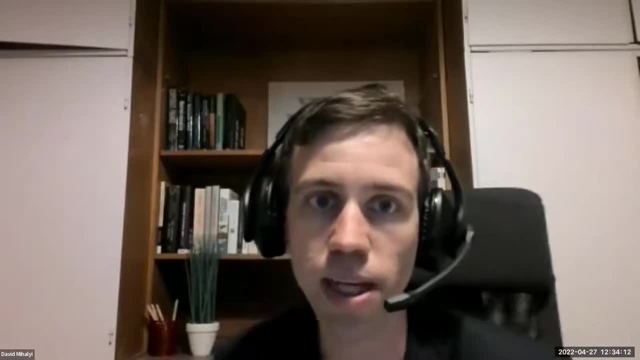 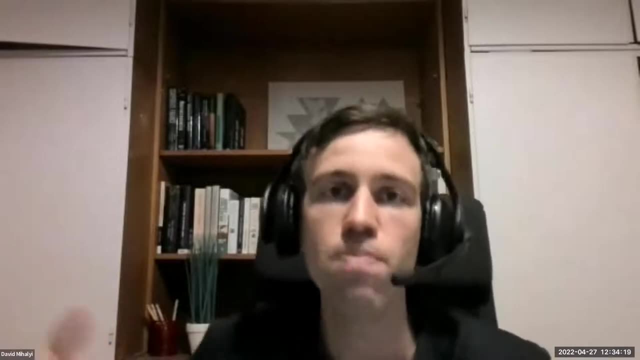 in a country to have you know a big chunk of the population. you know a big chunk of the population but it's very rare in a country to have you know a big being employed in the oil sector like a sizable one. uh, that's that's, unless you know it's through. 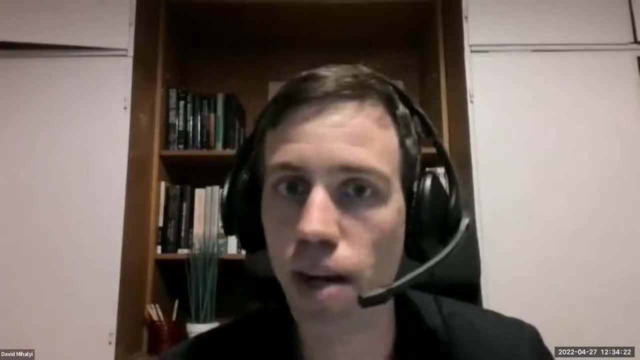 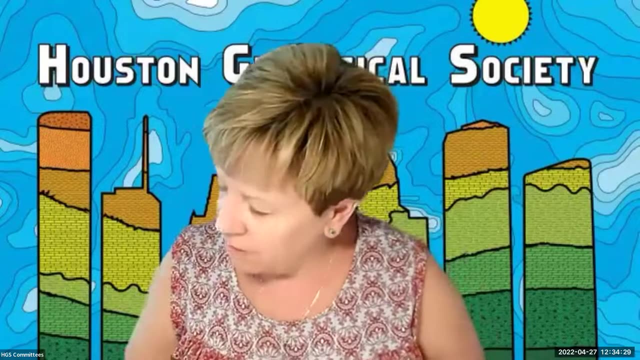 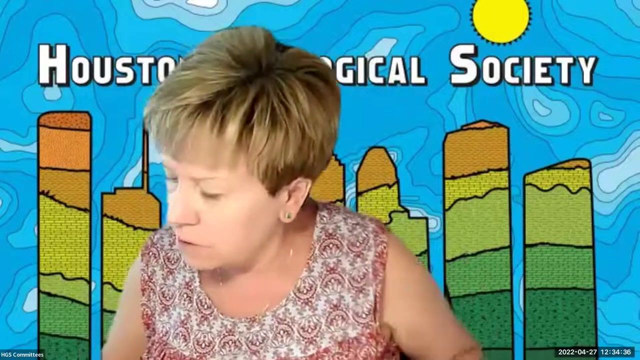 midstream and then right, but that happens a lot later than than you would. um, so, yeah, that would be the hypothesis that was. that was very, very surprising for me as well, and um, another question i had was on your timeline chart, which i thought because i was about to ask before you showed it. 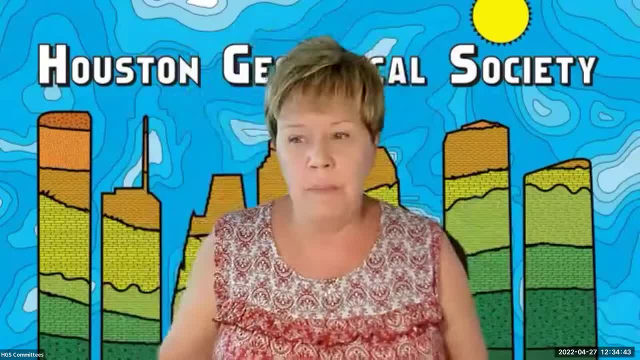 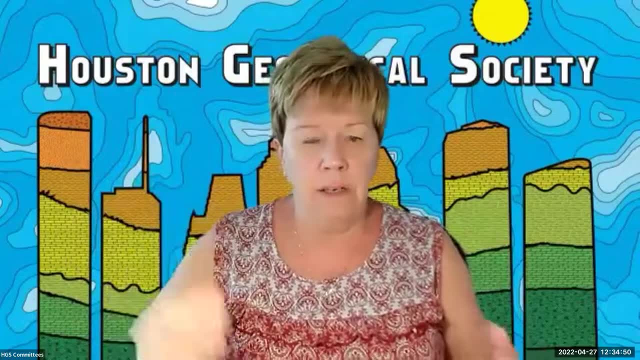 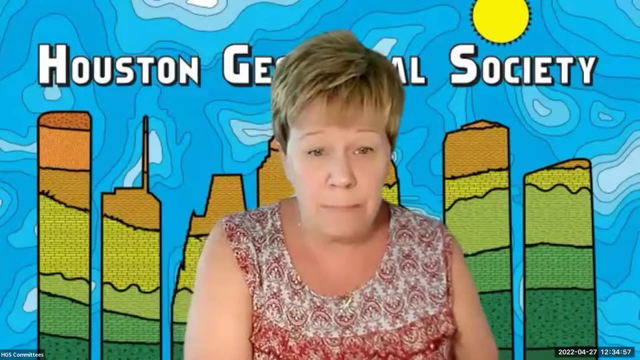 do you have this broken out by region, which you did? um? so when you look at that, because one of the challenges in oil and gas exploration is the fact that you know, until you actually get product out of the ground and it goes into either a pipeline, a boat or or a product, you don't make any money, right it's? it's, it's negative, it's. 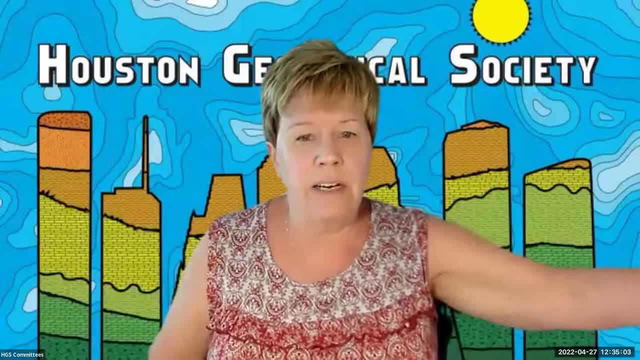 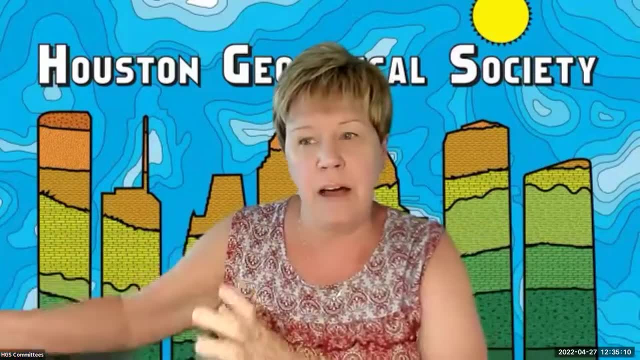 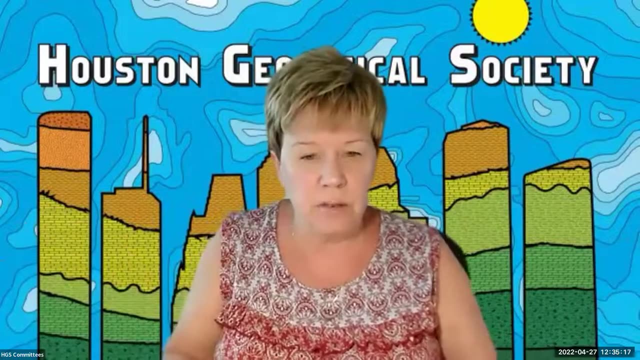 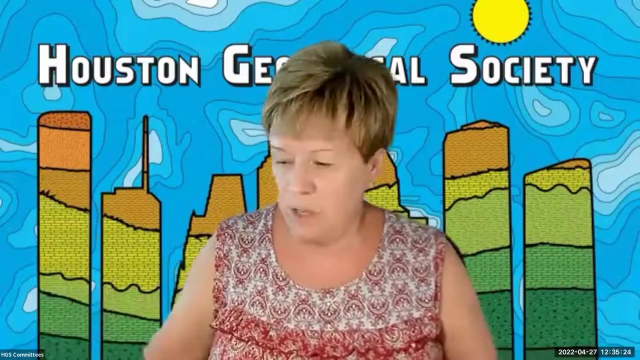 maximum cash impairment, and so in some of these countries it doesn't exactly it. it's almost a bipolar type thing. the countries that have a lot of remaining resources is where you want to go, but from your work and from your analysis, many of those countries are in places where it's an extremely long timeline to be able to ever get anything to market. so does 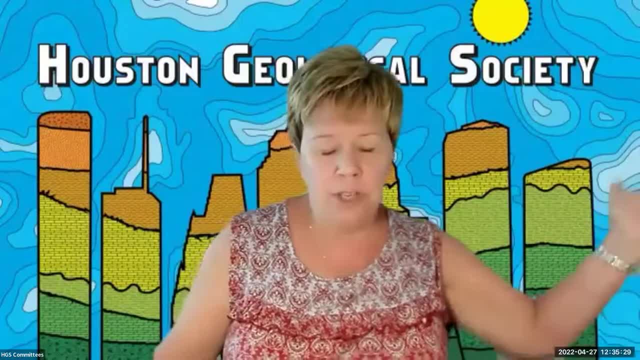 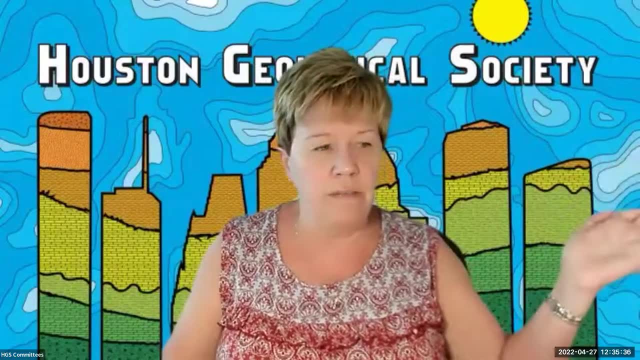 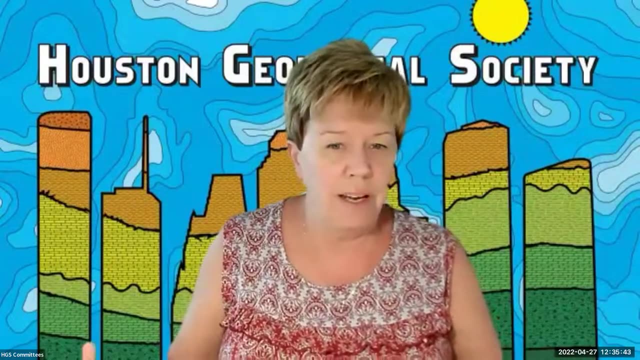 your chart. basically say: shift your focus to north america, which has less resource, or europe, because your odds of if you find something and getting something online sooner and making some money is going to be worse. better so it's. it's really a bit of a rock and a hard place with the data that you showed. 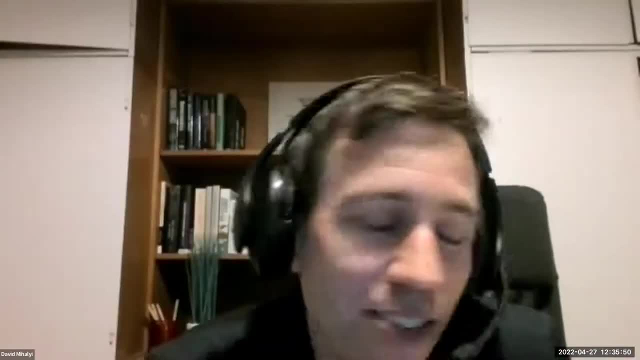 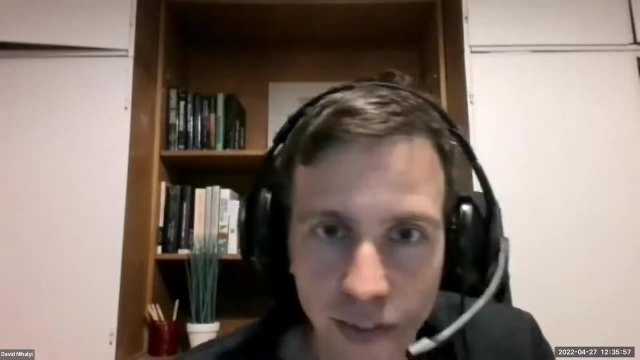 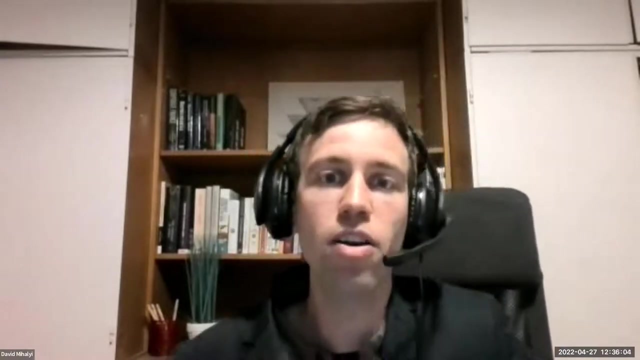 i've not thought of it that way, but you're, i mean, i guess that's. that's definitely one way, uh to to read, read the charts. i was thinking more from a government policy perspective. the idea is these governments need to fix whatever the problems they face. right, i mean, it's i, you know. 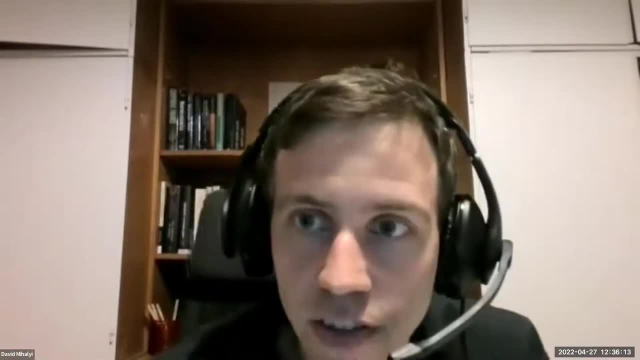 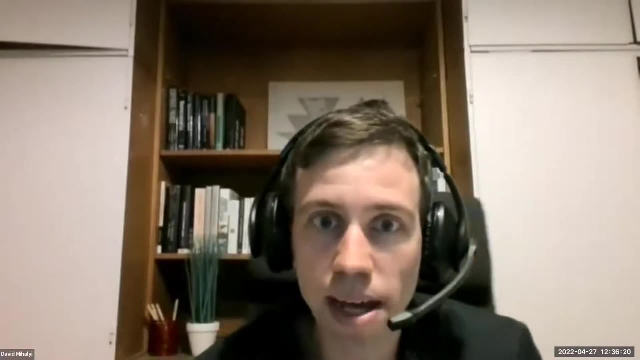 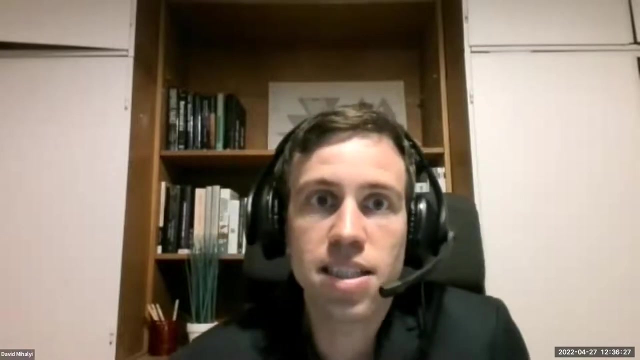 there's again. this is a golden opportunity now, with the world sort of craving for gas, uh, non-russian gas, i would say uh and uh and yes, and you know there's all that. there's all the gas in tanzania and senegal and uh other places, and it's just not not there yet, right. 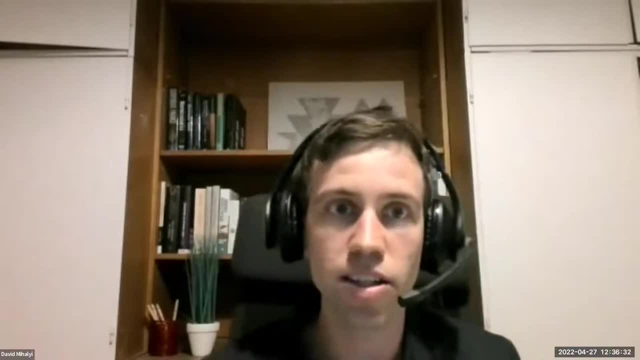 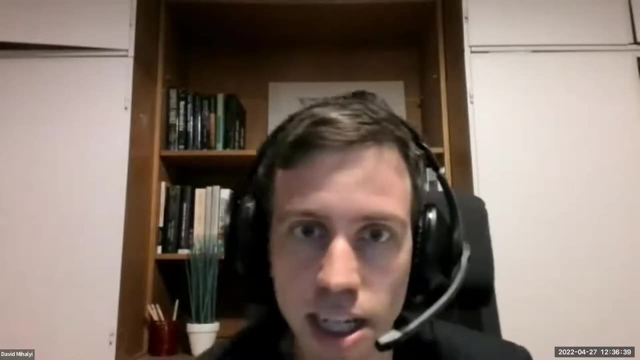 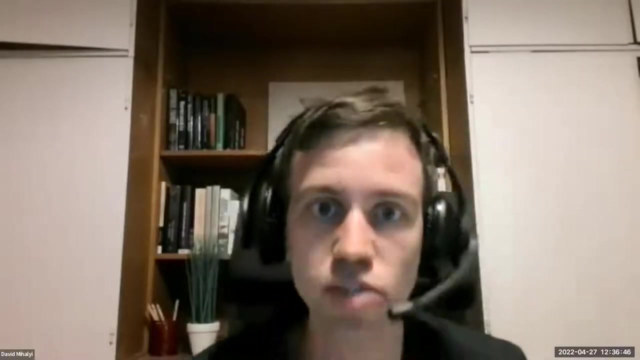 and, but it was, it was discovered a decade ago, uh, and, and you know, countries, uh, and there were. you know, i remember all the, all, the all, the controversies and negotiations, and in tanzania, uh, between the state, state ownership, domestic utilization, all of these questions came. 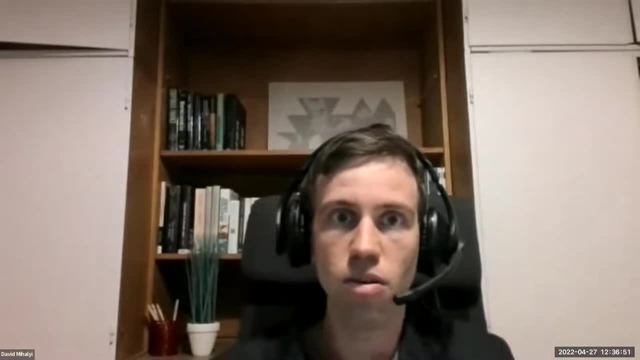 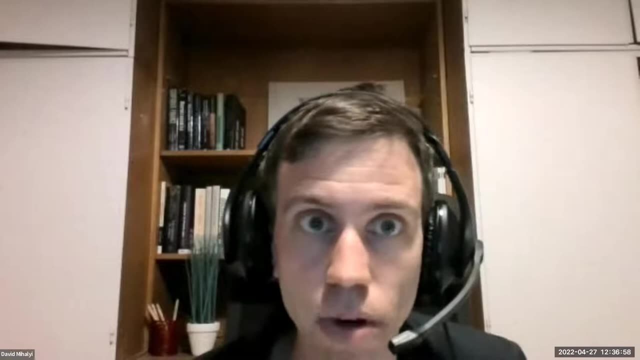 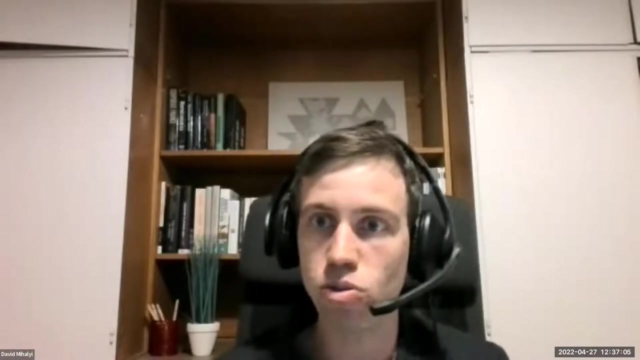 up and i'm not suggesting they're not important, but also there's, there's a risk that you know, uh, um, yeah, uh, that the indos and, you know, uganda finally secured a final investment decision like 12 years down the line again. it was those refinery and those, those questions were burning. 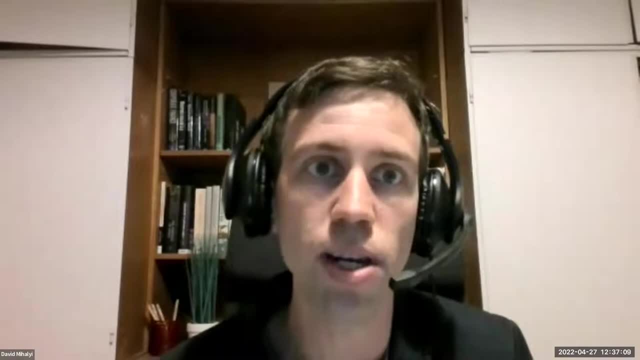 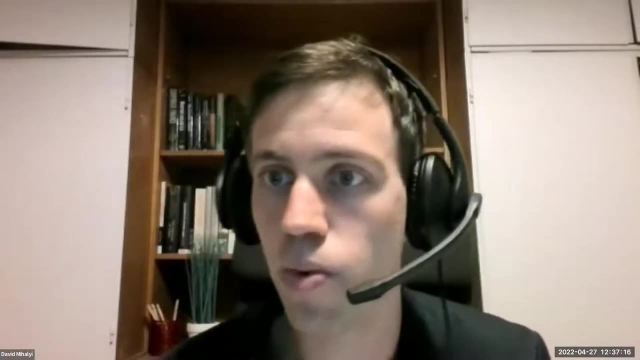 uh, so? so another way to read it is for policy makers to think through: uh, you know where, where those bottlenecks are coming from, and then, and what, what can be done about them? so michael hines has a question. um, michael, you can unmute if you'd like. 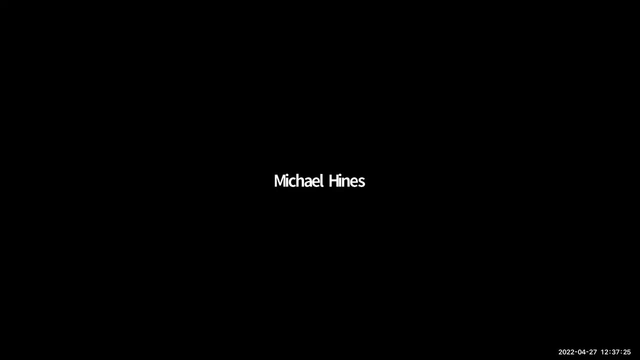 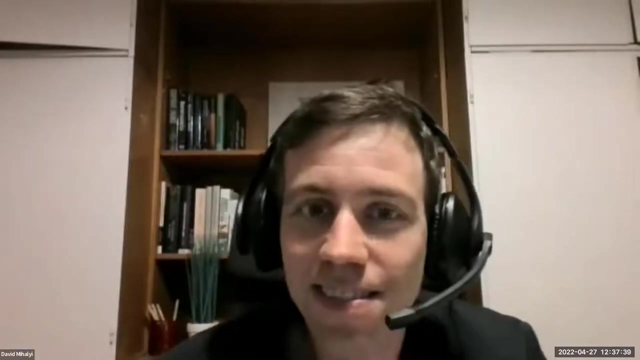 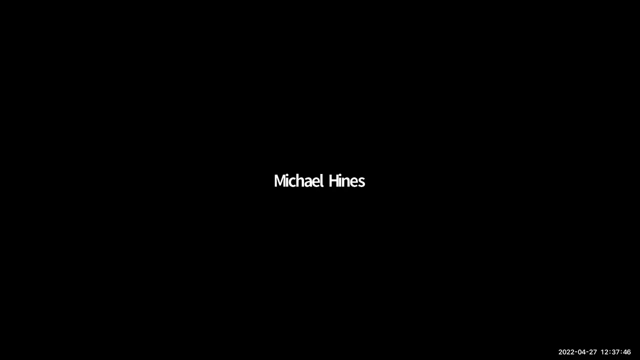 to ask a question yourself. uh, yes, hello, michael heinz. um, my question is: what can now be done to improve the much delayed african, to bring the much delayed african resources to market? thanks, questions. yes, they are delayed, but what can be done going forward? i think that's. uh, i like i'd say make clear, my research didn't really find like a magical. magical trigger where? uh, it seems to me one thing that i did find in data is actually domestic. national companies seem to be more aggressive, so nationalizations seem to trigger faster timelines. uh, not as in so more national, uh, national oil company ownership and and heart operatorship and all that. so that's not necessarily uh, so that that that may suggest. 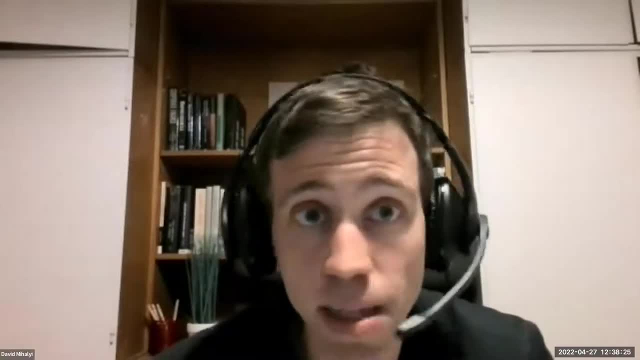 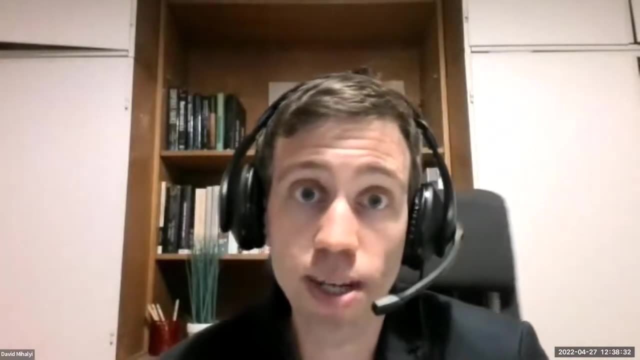 two things that may suggest that they are better at circumventing some of the administrative hoops, and, and, uh, that could be one way. or they're willing to take bigger financial risks. uh, because they have deeper pockets, because they know that the state's gonna, you know, support them. i don't. 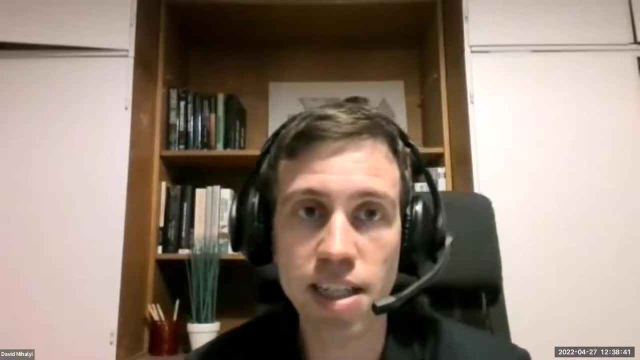 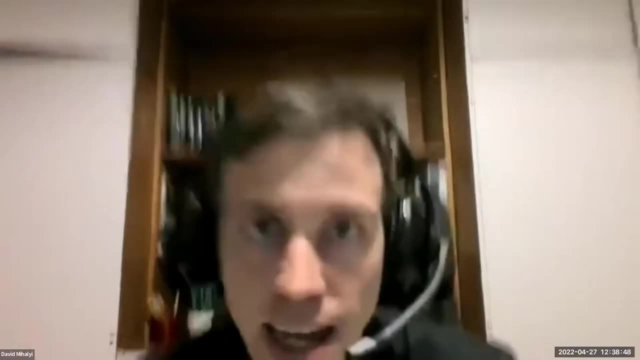 know. so that's, that's definitely one thing to think about. but, uh, you know, if you're like, you're like that the data suggested is that you know those with it. say, for example, within a country, the resources that had a larger NOC participation. 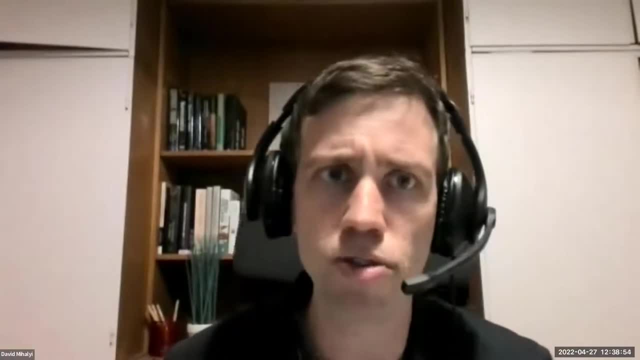 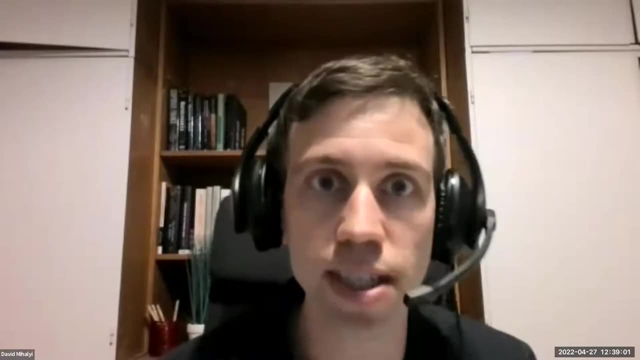 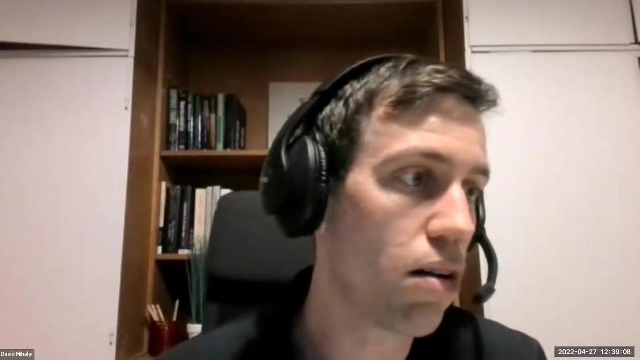 were getting these and you know most of the well. the US and Canada and a few countries don't have national companies, but in most countries there is one. So that's one part. I guess the second part is the harder one. 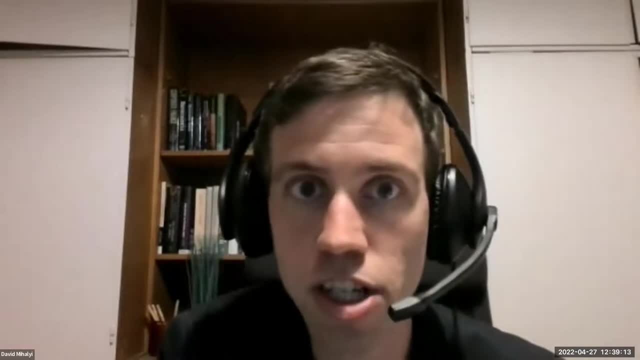 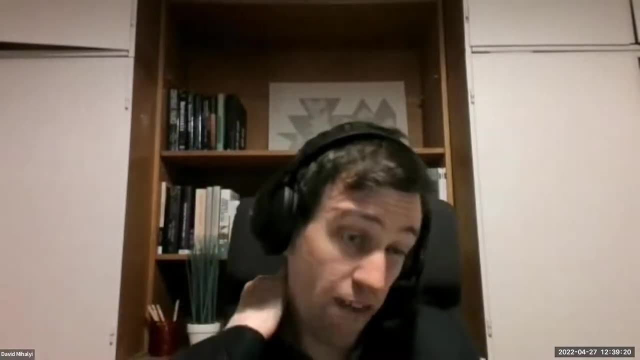 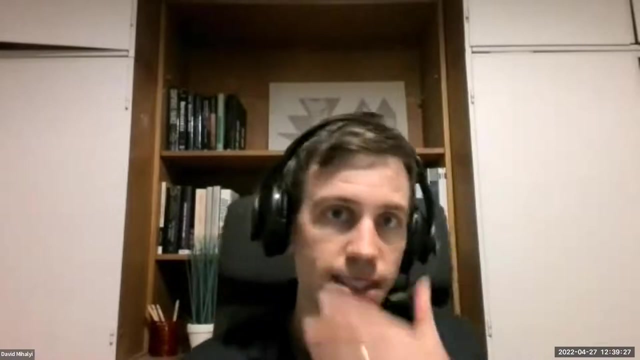 which is more about the types of institutional reforms and the types of procedures that should be in place. I think maybe one thing that I'm particularly interested in is the whole sort of local use idea. It seems like a sticking point in many of the countries. 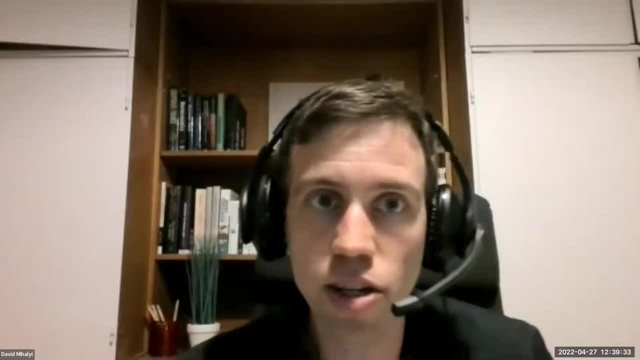 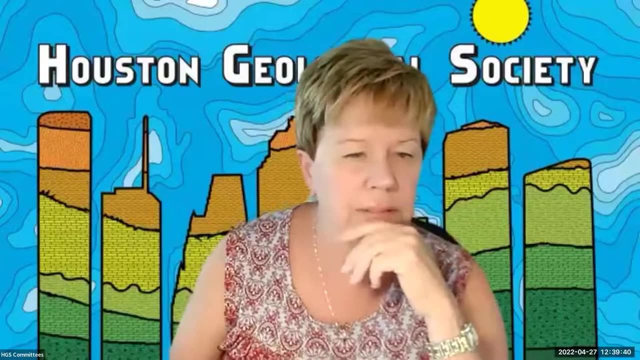 is that they wanna make sure that they don't just get taxes but they also get Local content. Local content or domestic utilization or other types of benefits. So I think that that would be an interesting question to research further, but I've not gone. 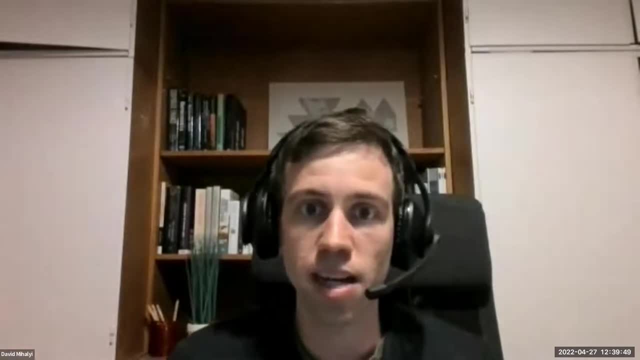 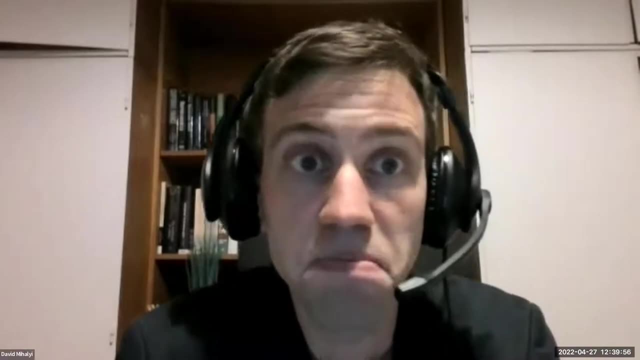 I can't find the data in a clean way which would tell me which countries has how much of these obligations in a way that could use that, But I think that might be one of the avenues to look at. Yeah, it definitely speaks to you know. 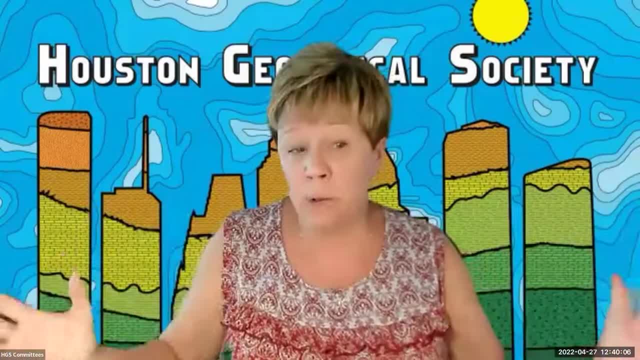 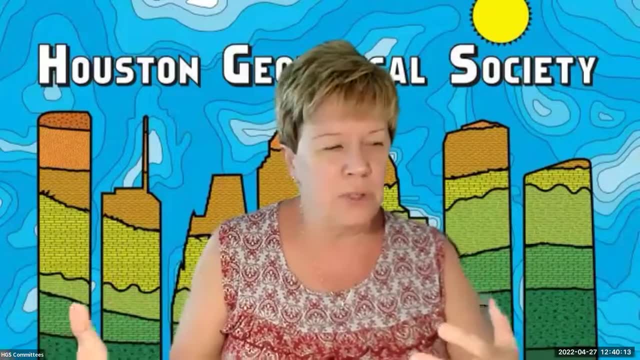 as geoscience experts, you know as geoscientists, you know we follow the rocks right. So you know it's difficult at times when I would work with our commercial side. our commercial guys would be like: 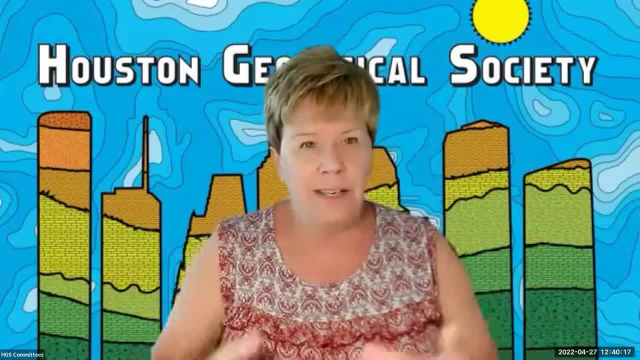 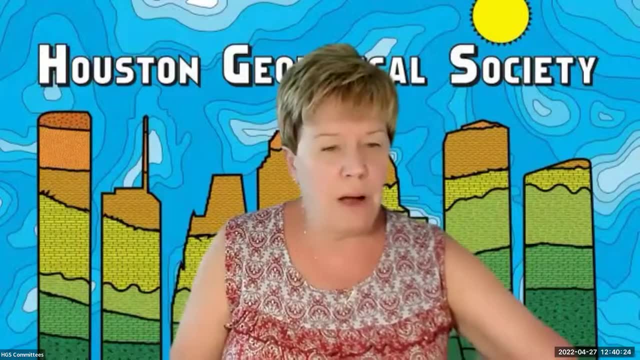 well, why don't you guys just go to these places that have the best terms? It's like, well, having the best terms necessarily mean you have gotta start with good rocks, good rocks and good source rock, Which is what is so sad about both Mozambique and Tanzania. 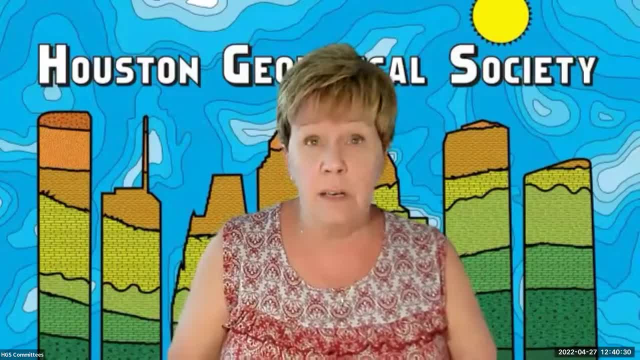 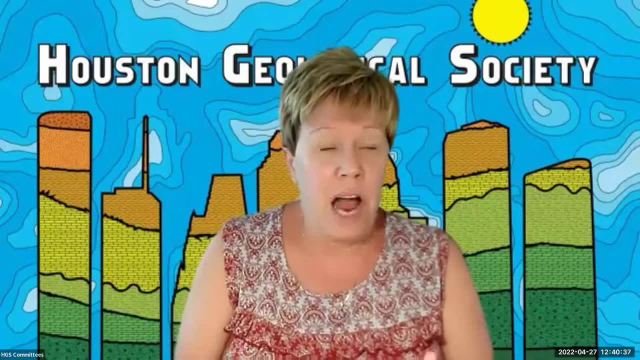 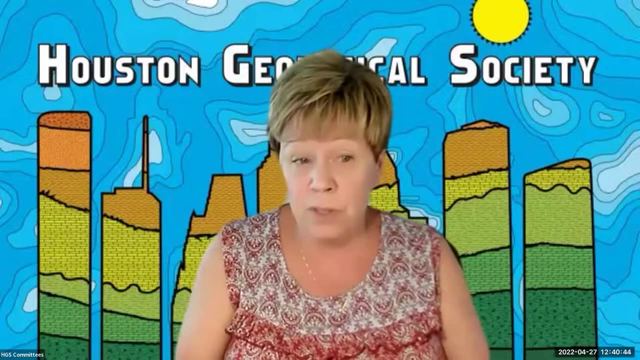 And I've seen the data from both of those discoveries: fantastic beautiful rocks, fantastic Fantastic resource, just challenging in a country that kind of can't get their act together to make it happen. And you had three majors in there trying to bring these resources to bear. 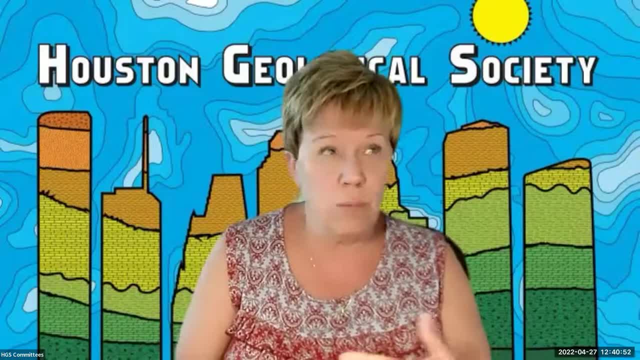 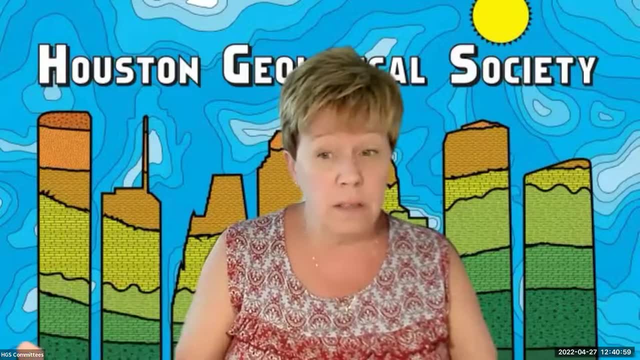 and you just couldn't get there. You know they're in deep water, they're gas, So there's those challenges as well, but really really tough, you know, and all the discoveries in the Romanian Black Sea were similar as well. 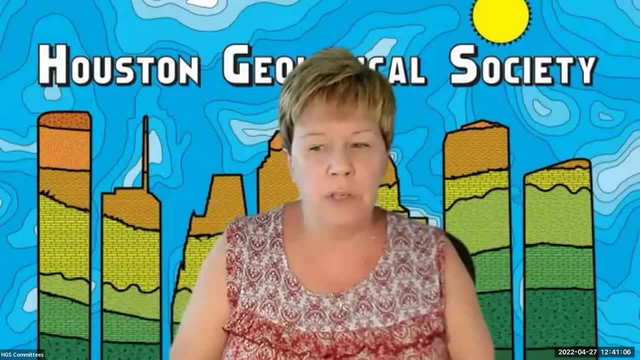 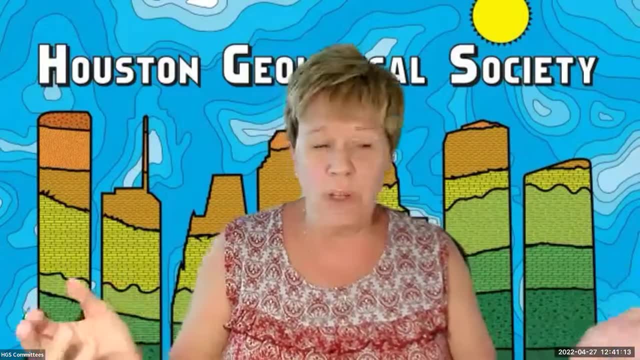 Beautiful resource, But just very difficult to be able to bring forward. So it is a real challenge. So you know, as a geoscientist, if we're like Doctors Without Borders, right, It's rocks without borders. You just have to go where the best things are. 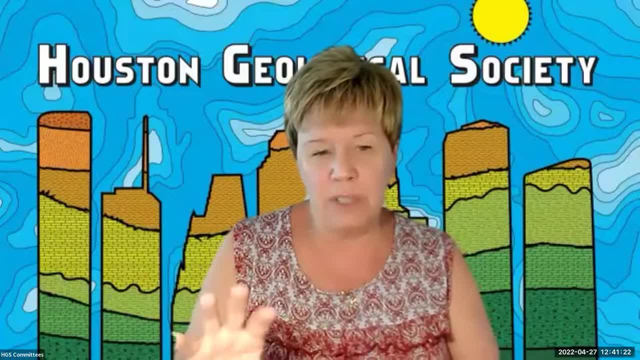 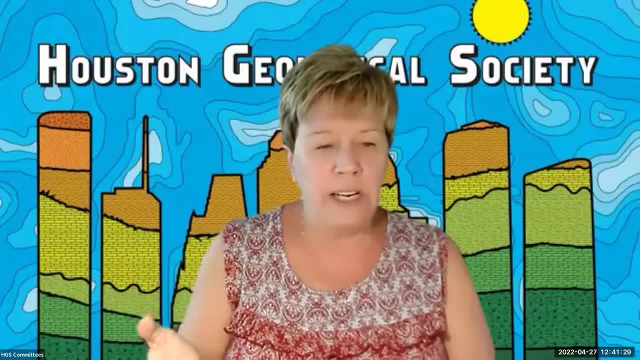 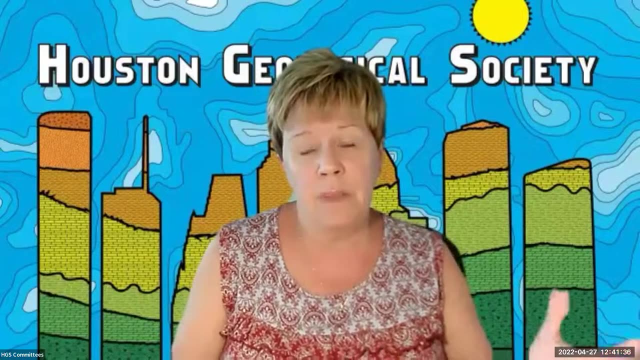 and then kind of hope for the best. But your data does bring up the challenge of, especially in the current investment environment. if it's 10,, 20 years to bring something online, that's really really hard. So that comes back to the 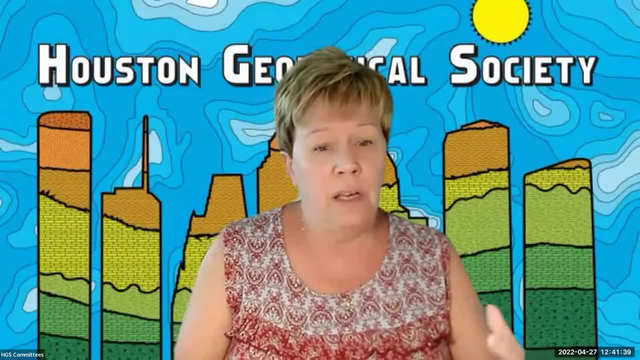 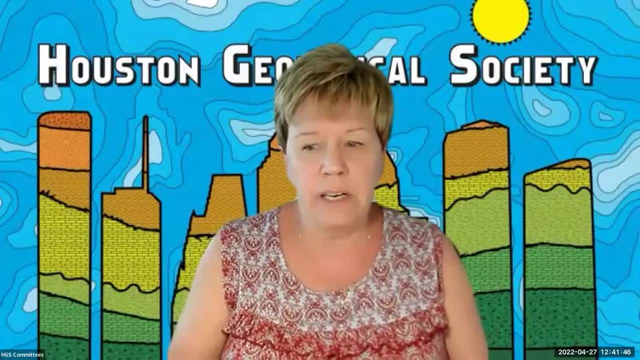 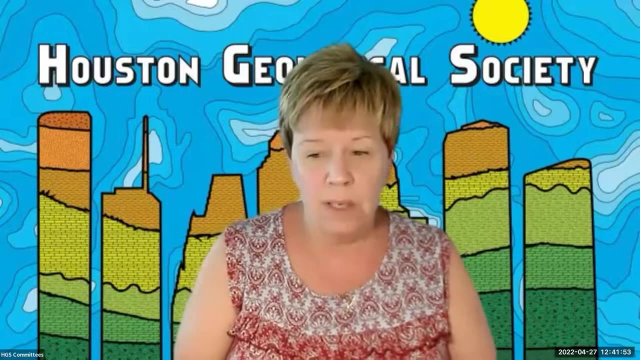 do you think your data is showing you know you need to do more with the resources you've got, like back to North America, or is it enhanced recovery? Is it other things, Even though the US isn't necessarily seen as a really good, stable regulatory environment? 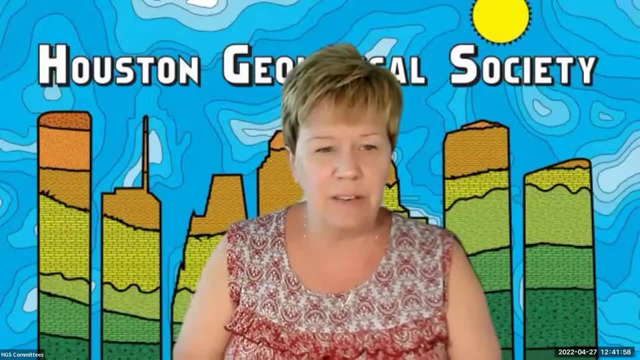 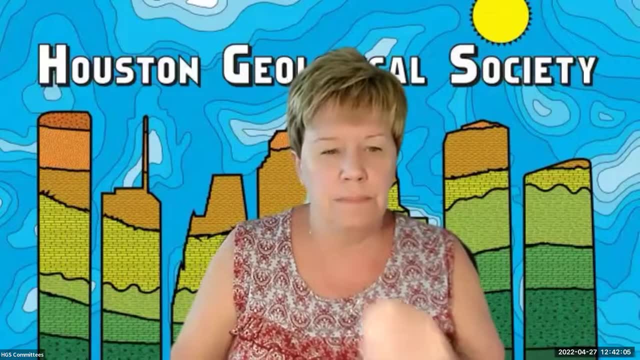 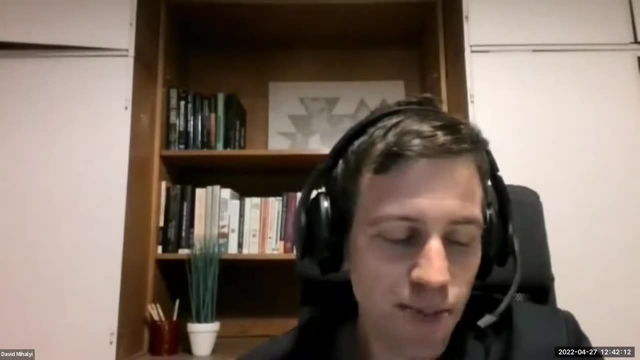 because it changes a lot, but at least you can get stuff going. It just points a really challenging picture and a challenging conversation. It's a conversation with non-industry people. Well, you know, geologists follow the rocks. I mean, my co-author, Jim, has another paper. 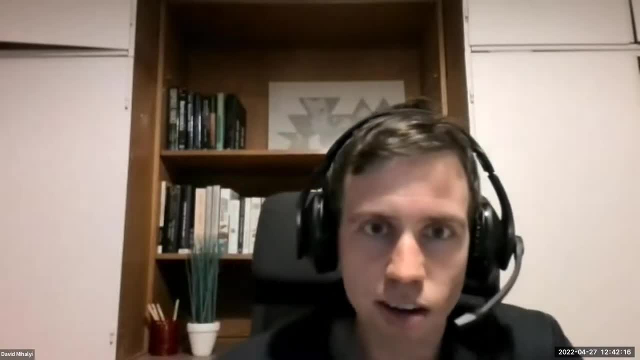 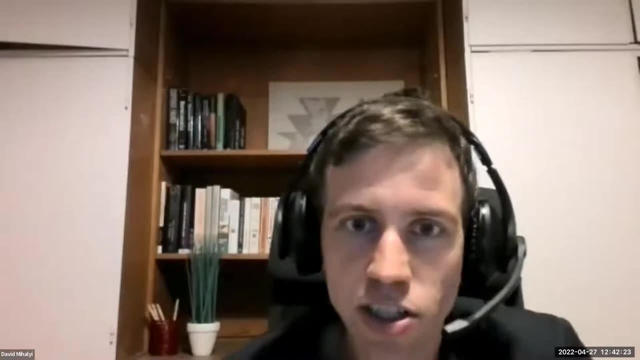 which comes to mind where he looks at drilling, so exploration near borders- And he finds that, you know, like if he looks 30 kilometers left and right to the border and what he finds is there's a lot more drilling happening. 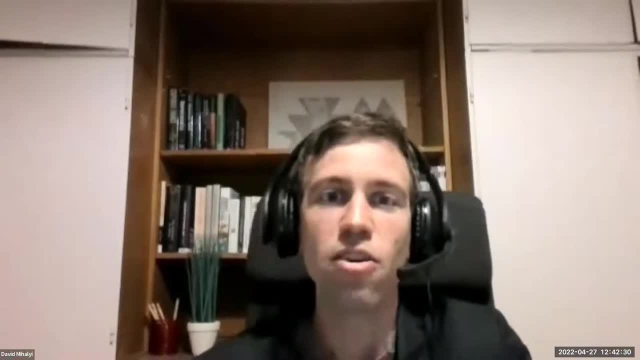 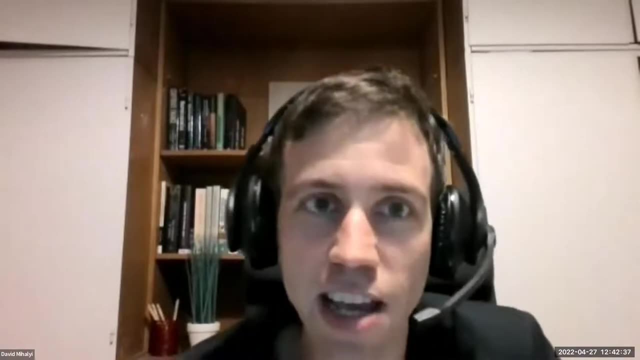 in the country that has these better institutional and governance scores, right. So yeah, I guess from a geologist perspective, 30 kilometers varies little, but if it means that you're on the other side of the Mexican, you know, US or the whatever border. 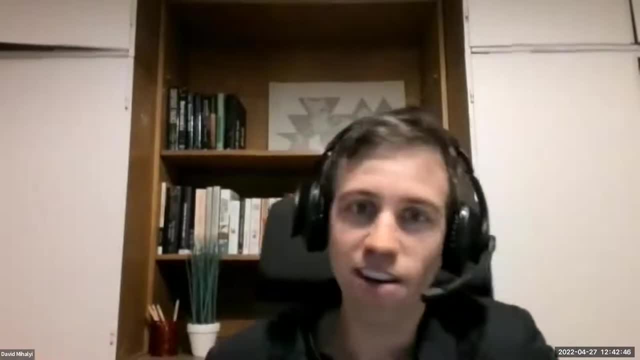 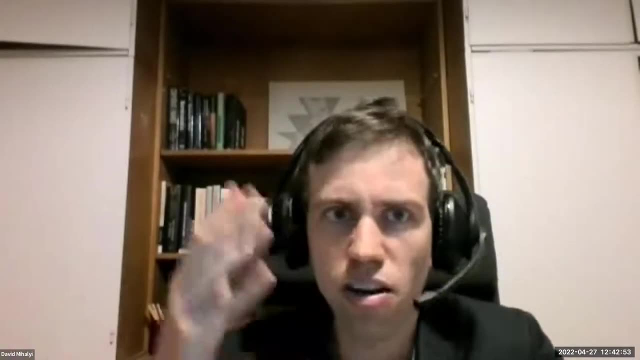 and you can choose the better regime in terms of whatever it could be, you know, institutional, anything, any of those elements. then you know, you see these patterns, and there's the Uganda DRC line and there's a lot of these drillings. 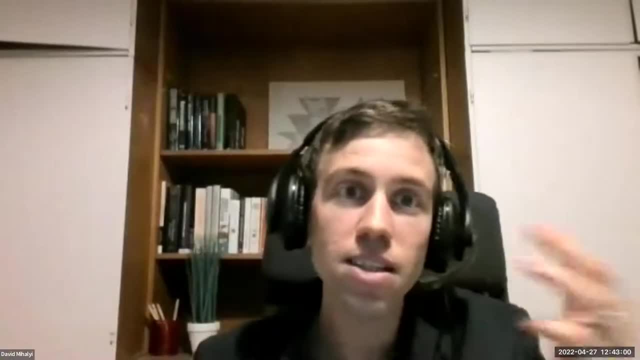 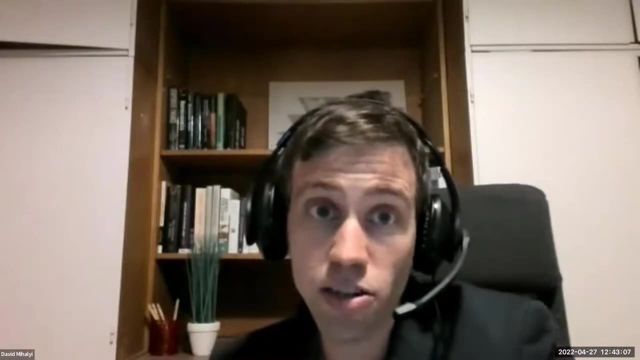 that happen very close to these border areas. So yeah, So it's. I mean, that's definitely part of the story there, And I guess part of the reason that so many of these countries found so little actually is because no one had really explored them, right. 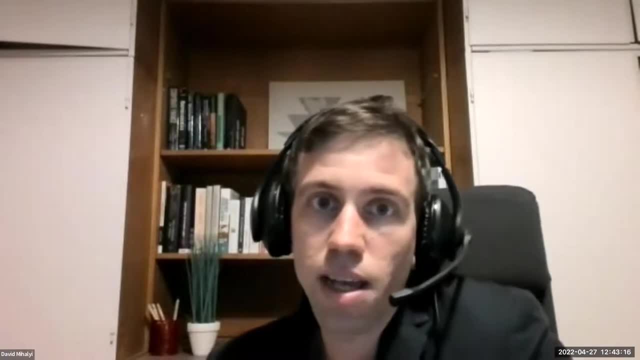 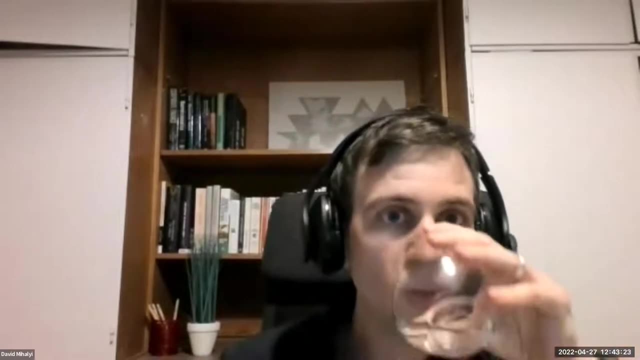 I mean still Africa's way less explored in terms of the amount of exploration drilling that happened compared to, you know, North America or whatever. There's an interesting chart you can pull up So when you guys further your resource, if you also look at. 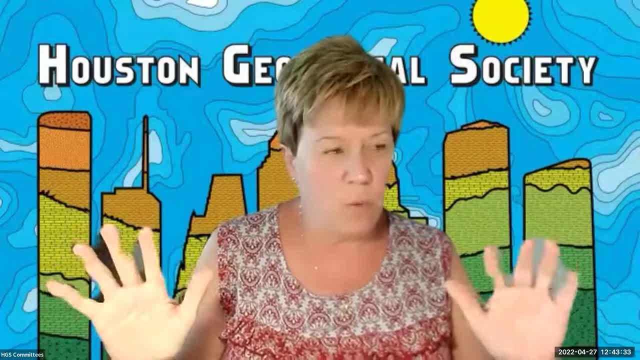 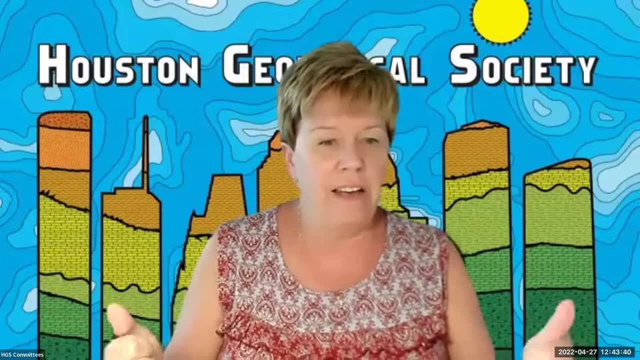 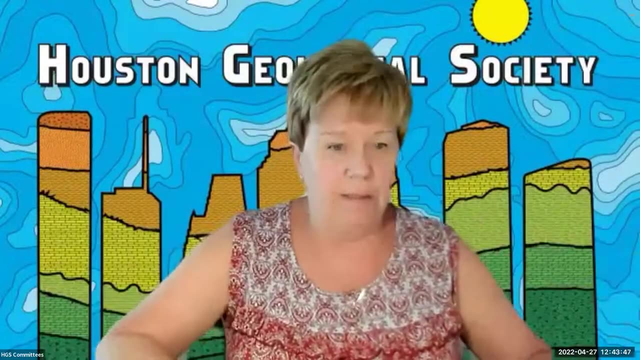 because we had this chart for a while, the amount of seismic that's been shot right, Because seismic is always our precursor to drilling And you can pull up from public domain sources essentially what the Africa continent. it's more offshore than onshore. 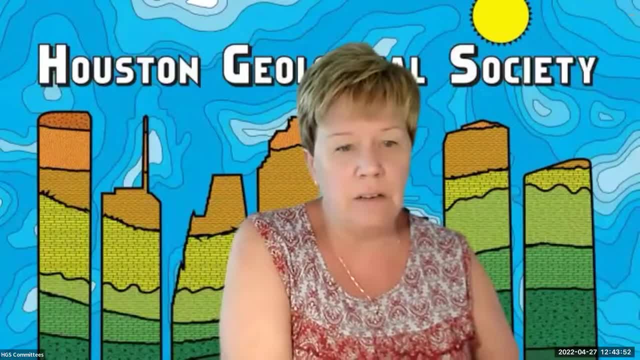 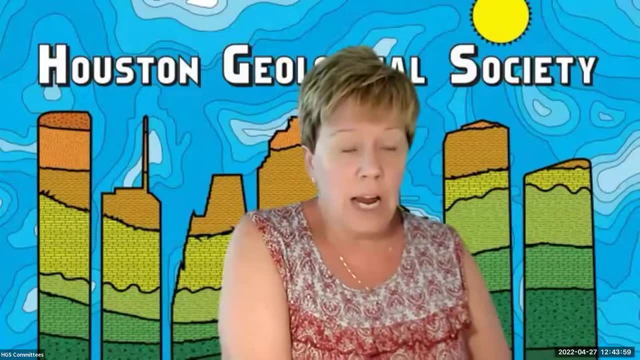 It's harder to pull up the onshore, But what that looked like in terms of seismic coverage in 2007 and what it looks like today, and it's it's incredible. There's very few parts of the Africa, And I mean, what's all the way around, right? 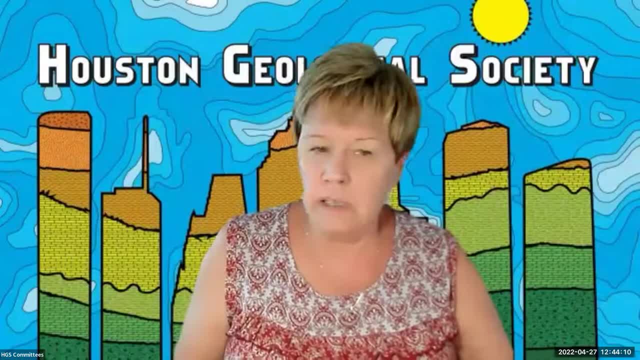 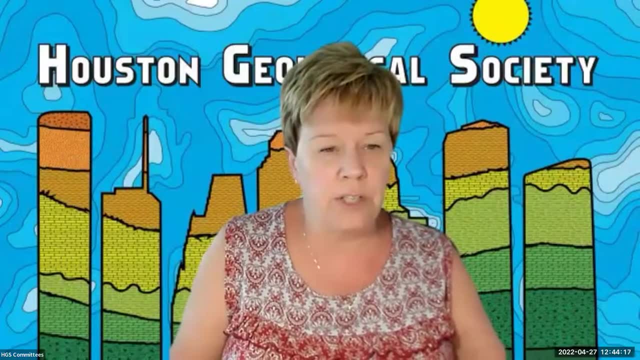 That is not currently covered by at a minimum 2D and sometimes fairly dense 2D and a lot of 3D data. So sometimes the amount of drilling is done, it's done as not a reflection of how good that country is. 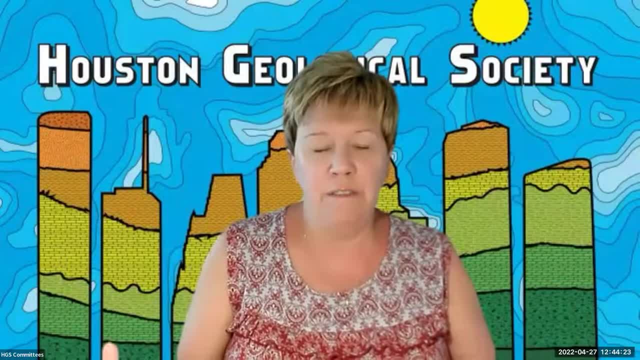 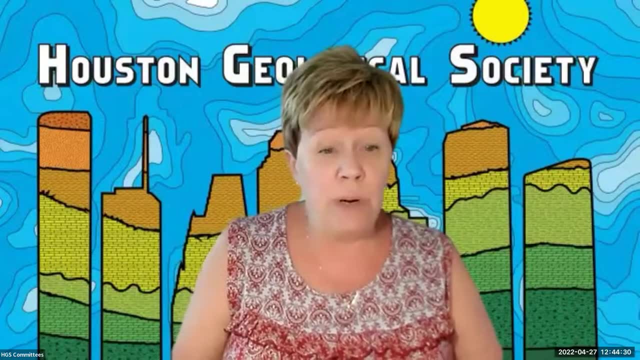 It's okay. where's all the seismic been shot? And then, if you look at that in relation to what countries think, because it's kind of scary when you go out there and you look at how much money has been spent, In fact, Joe Riley, when he does his talk at the end of May- 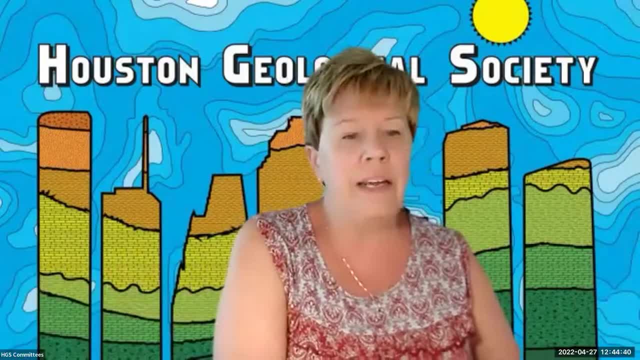 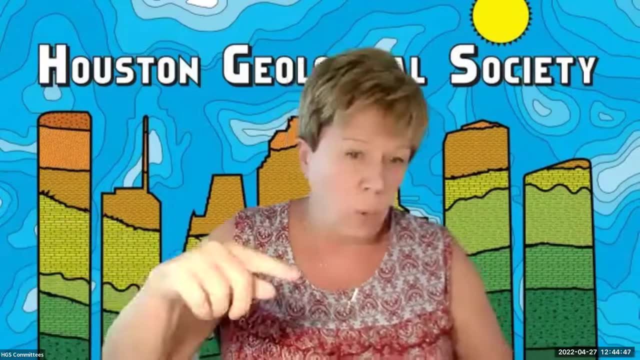 he's going to talk about that. when you look at from the 2D to the 3D and the rush now to find more stratigraphic traps around the globe, which started with the success in the Alvorean coast And then now, of course, Guyana is the golden child. 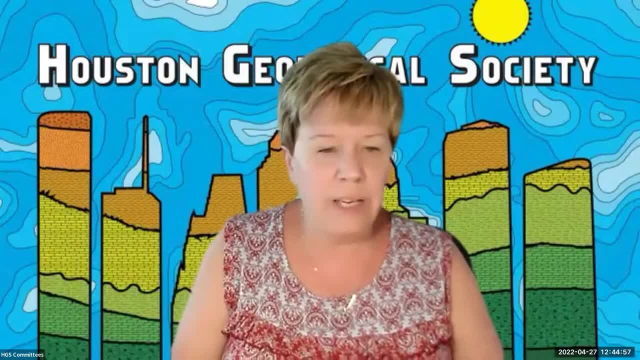 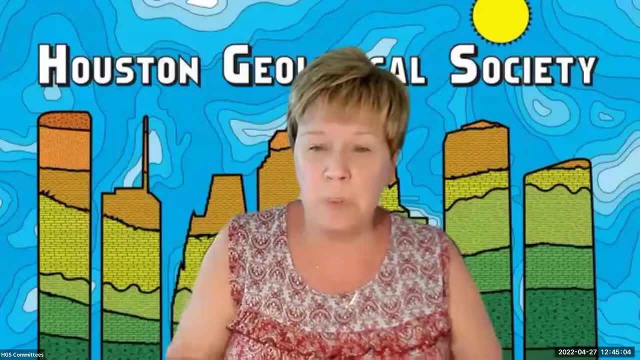 There's a lot of money that's been spent on data. So yeah, it's. it's definitely going to follow up on the on those charts. I've not seen the. the seismic- Yeah, the seismic one is pretty telling when you look at what people have done. 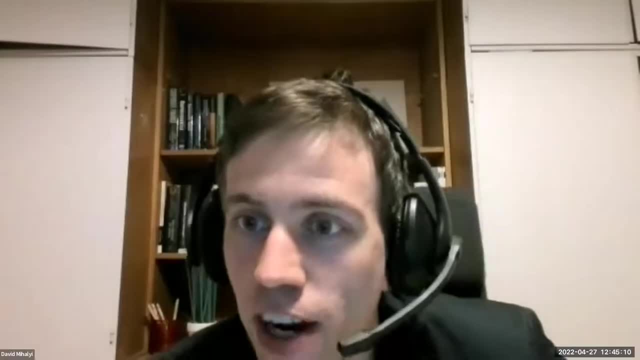 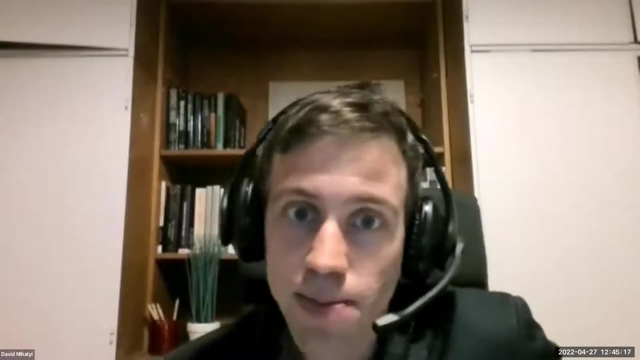 Michael has another question. I think it's a comment about overlapping claims. Yes, I've seen the there's a lot of resources in the disputed territories, or well, sometimes it's it's resolute, you know it gets resolved. 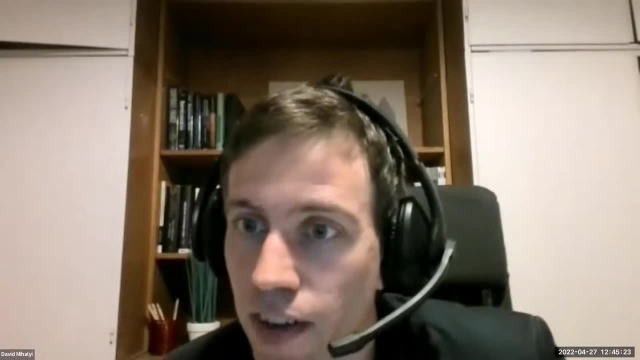 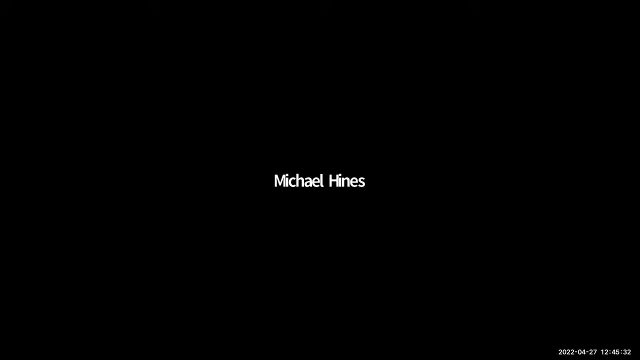 Yeah, Yeah, Yeah, Yeah, Um Of northern Iran, but it's very extensive in the South China Sea. Right China claims most of the offshore to China, Venezuela, China, Vietnam, China, Philippines, you know. so the deeper water, 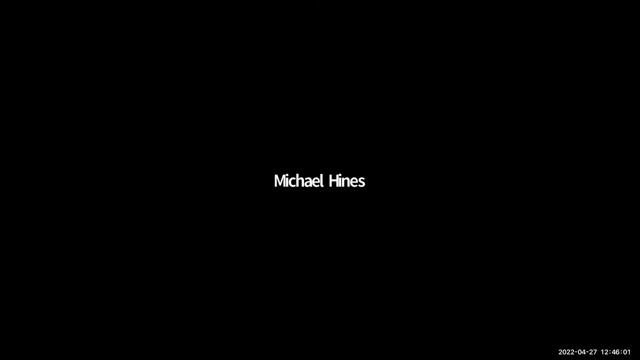 of all those basins has been severely reduced and it leads to a complete hold, as you quite rightly said. it prevents any initial lock, any seismic shooting which prevents exploration, drilling, which prevents appraisal, which prevents development. you know, it goes all. 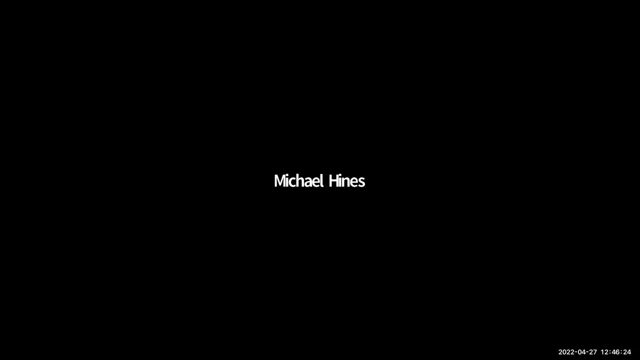 the way through the cycle And without mentioning any names. my old chief exploration manager used to have a map of his world and he had three types of countries: countries with good rocks, countries with good politics and others. For him, it was at least as important you. 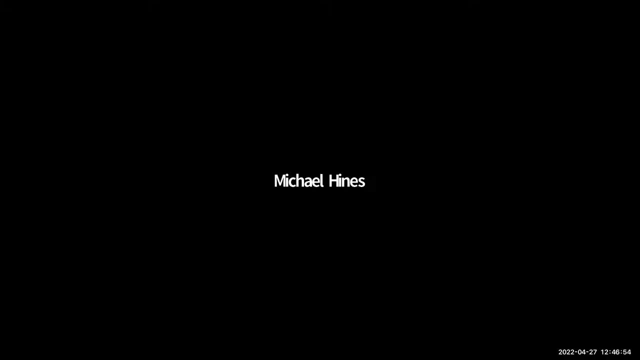 know there's such a, So that led to many countries being simply off limits. You simply wouldn't do exploration there, even though you knew there's lots of oil, but merely that's technical oil that has no value to the company, Unless you can produce it profitably. it might as well you. 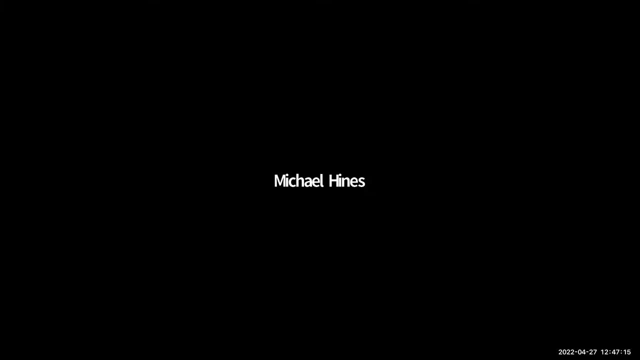 know not be there. Yeah, Michael, that's a great point, You know, Yeah, And in the real world, seeing we work for commercial companies, most of us- it's usually a high level filter that's put on by management that selects out which country we can enter. 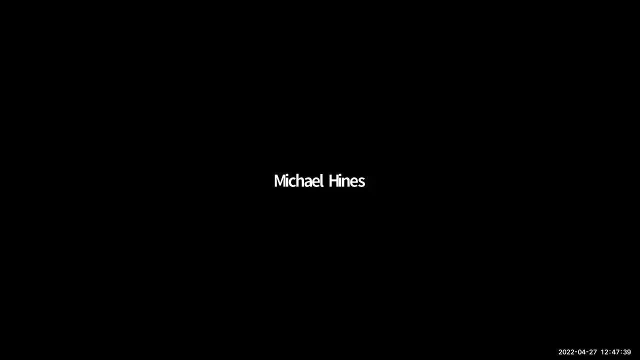 and which one we don't. And we're seeing a massive example at the moment in asset loss in Russia to many of the majors. I mean, those assets, I think, will simply be lost and they will be written down, Yeah, And they will be nationalized by. 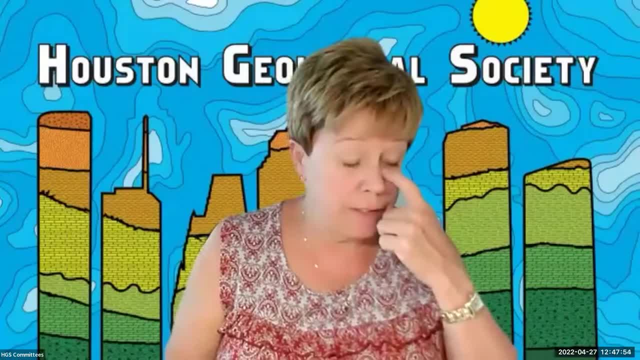 Nationalized by Gazprom, Gazprom and Rosneft, Yep, So it really does matter this political viability. Let me follow up on that. Actually, Michael, I have a question to you, I guess, on these. Well, you mentioned, obviously Gazprom may be taking over some of the assets within Russia. 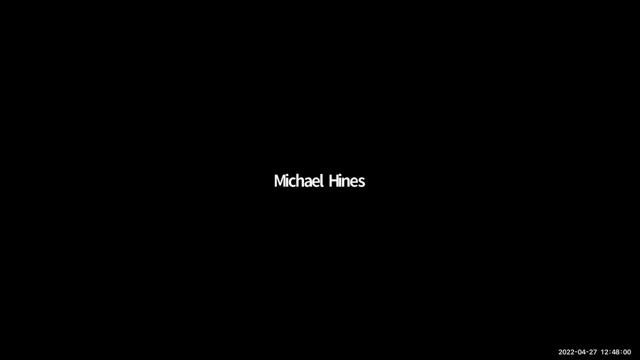 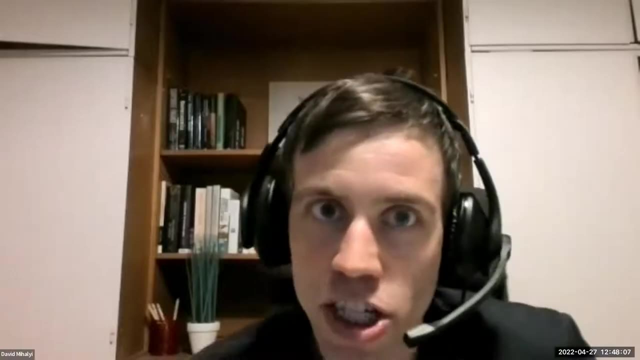 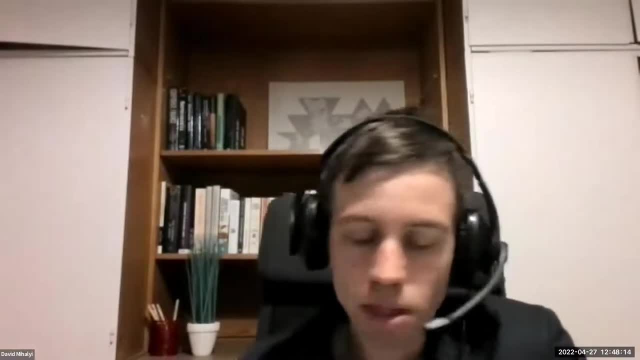 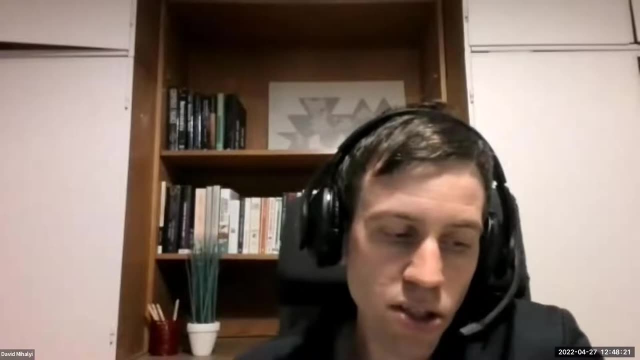 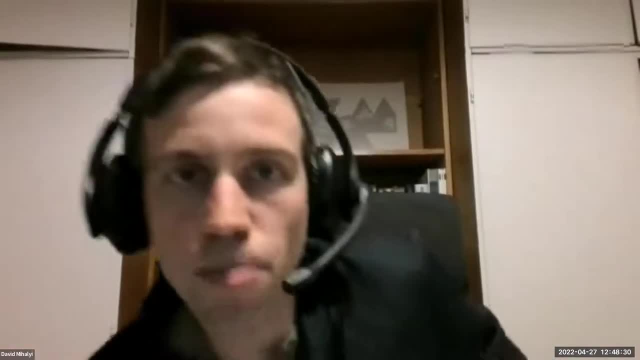 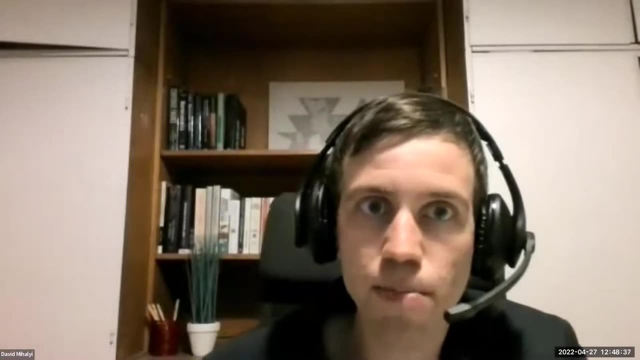 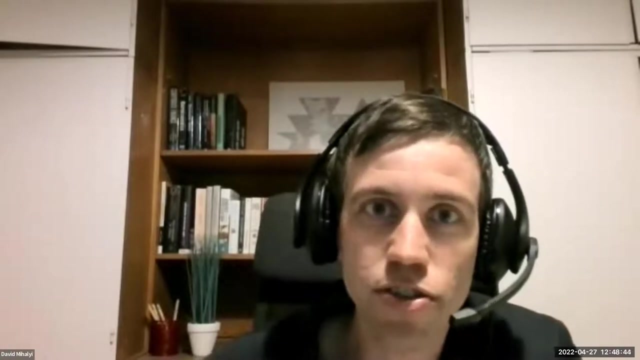 these companies? they're- I mean Petrobras at least- is probably listed, but like these companies, they're mostly nationally, at least majority nationally, owned. Are they more aggressive in pursuing some of these opportunities in what you call politically risky but geologically good countries? 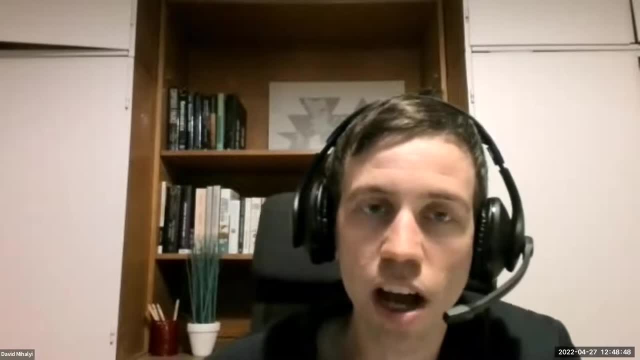 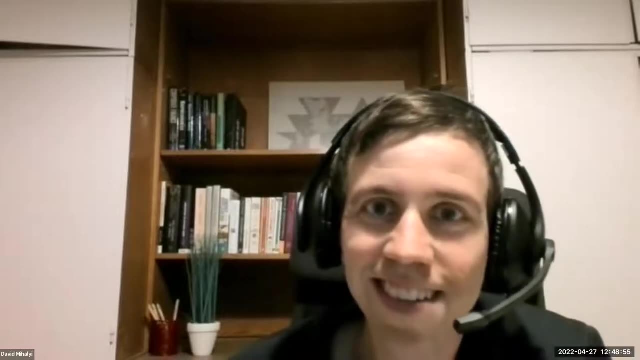 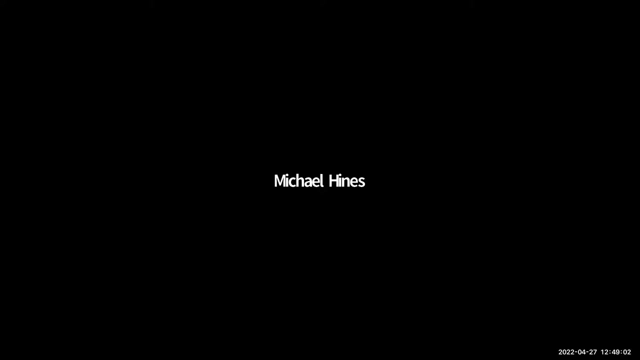 And do you think that they might be? they have a higher tolerance level for for that kind of political risks. Is that how you see it? or Yeah, I think they do have a higher tolerance for political risk because, unlike purely private companies, 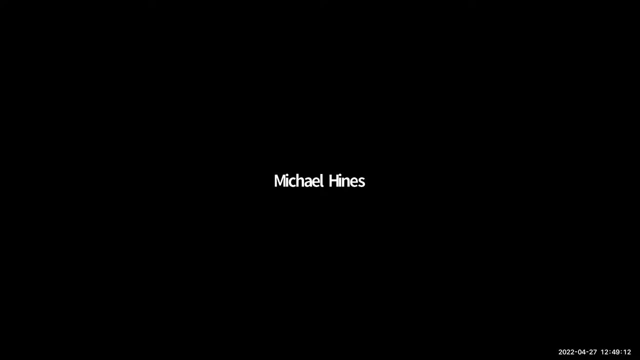 which have really no influence in the political sphere. national oil companies are a branch of the government and therefore they can act through their government to influence another government to take certain actions or not take certain actions. So that's why they have, you know. 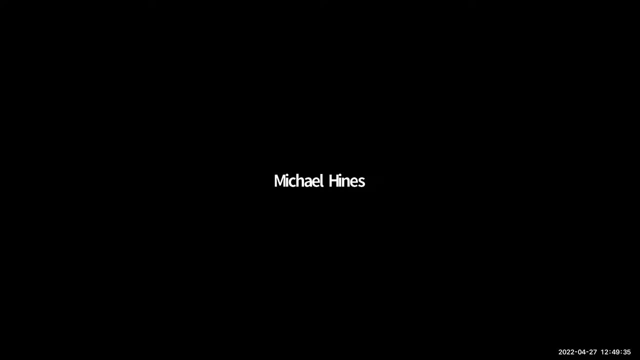 if you like, a greater ability to work, often with other second and third world countries, And many of them, many of them, are themselves located in second and third world countries. They are the national oil company of Nigeria or Malaysia, or I would say Russia as well. 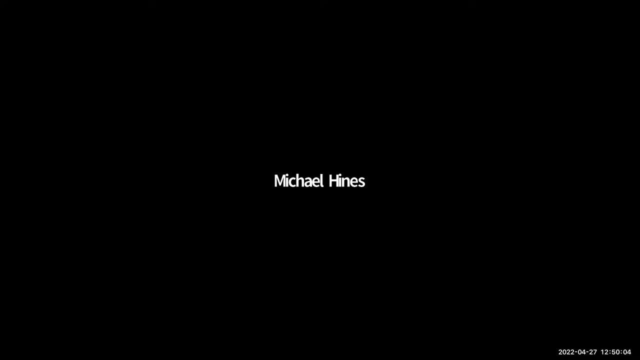 And so they see themselves having a different, different role. And also, when it comes to justification, they can say legitimately: we're not just interested in making a profit, but we're doing this for the good of the people of the country we're from. 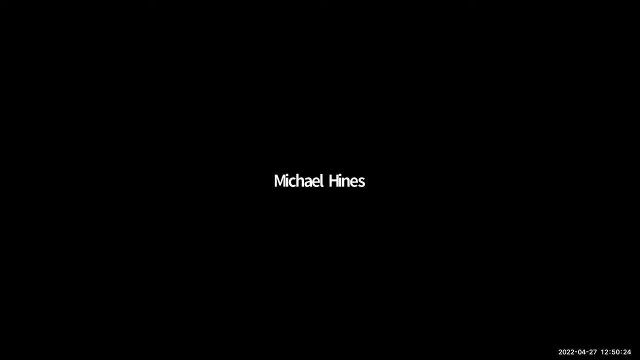 and the good of the people we're trying to do business with. So they've got a lot- they think a lot- stronger hand to be able to influence things And so can effectively be more, you know, more- aggressive. I mean the past masters. 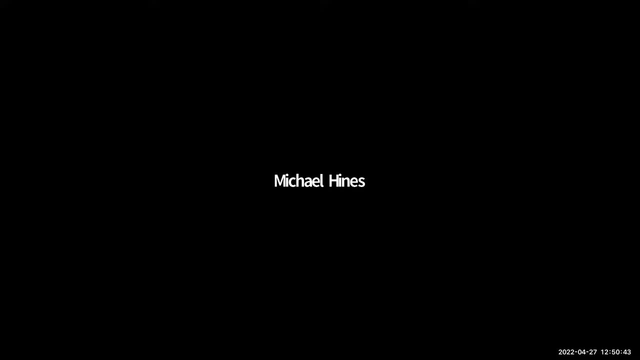 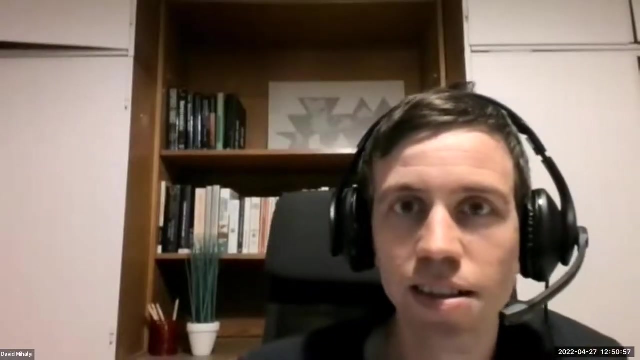 depending on how you look at it, are the Chinese. globally, They are the, and often the deals are not purely monetary based as in the Western IOC model. They have, like these bar trade deals and all that Deal to the whole country and they'll build railroads and steelworks, you know. 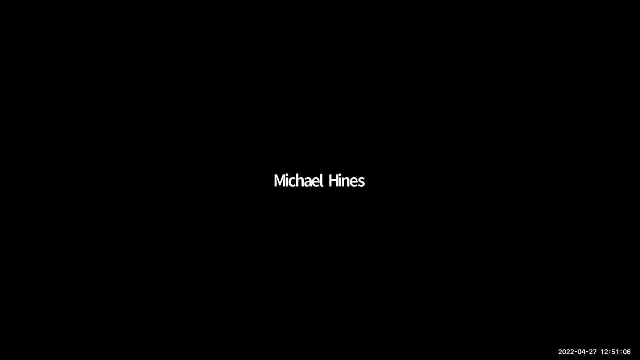 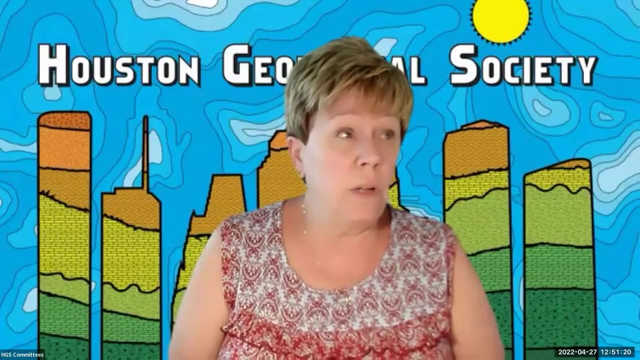 So they just see it as a part of of many other things. So many Western oil companies won't compete with that Absolutely, Yeah. Yeah, I mean, they do exploration as well, or they do like. Nexon is owned by CNOC. 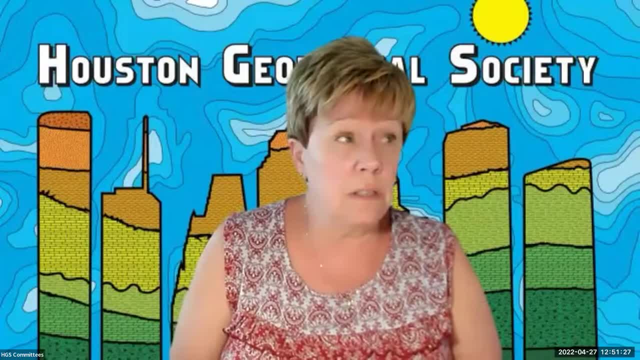 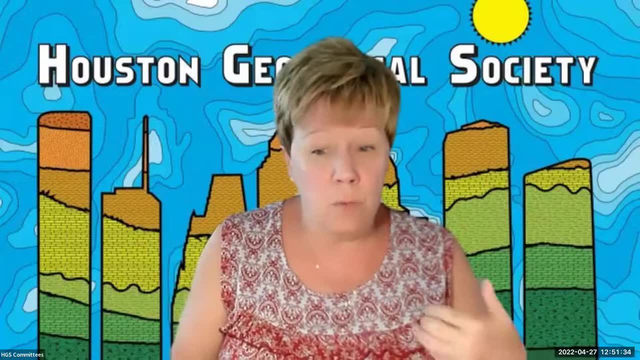 which is a Chinese national oil company, And both CNOC and CNPC several years back stated they wanted to be more of a global player, which is why they are one of the partners in the Sabre block with Exxon Mobil and Hess through Nexon. 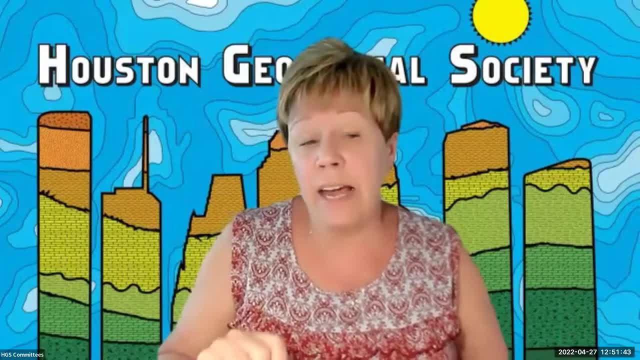 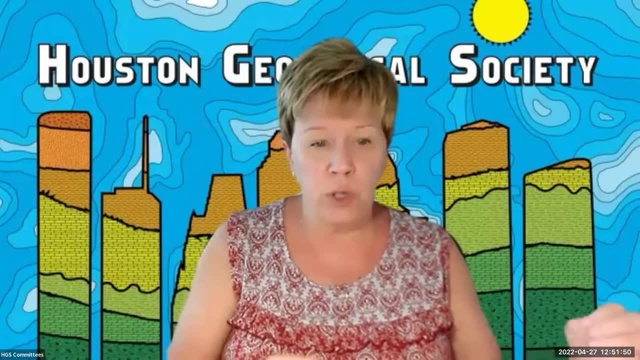 They're kind of US affiliate but they do, But typically more in exploration as a as a joint interest partner, not an operator, even though there's a lot of places now where they're going in and they want to operate as well. 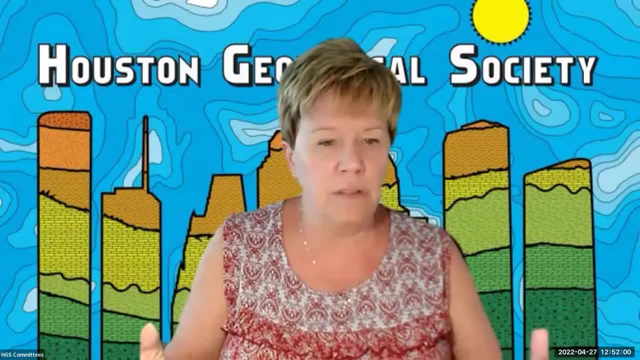 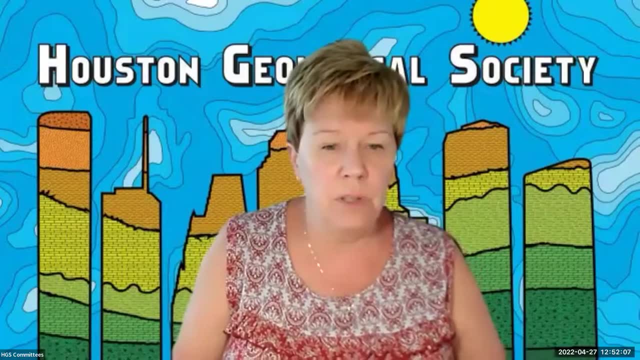 So it's as Michael was saying. it's this: establishing yourself as a not just a national oil company, but also a true global player with your own reputation. So it's a bit of a compete with, Yeah, And did you see that last week? 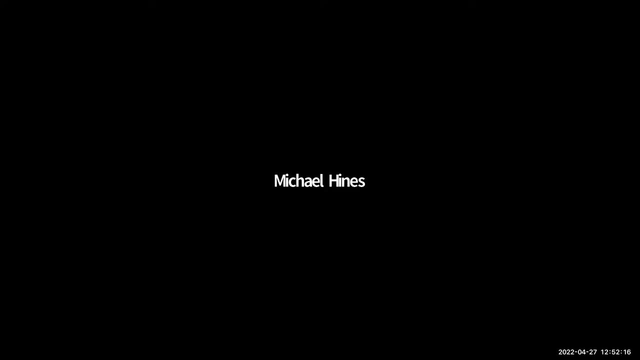 There was an interesting announcement from CNOC that they're actually exiting their Western countries position- US, UK, Canada- because they want to pursue this strategy of essentially third world targeting. Well, there's strategic advantage in that area, Yeah, And they are. 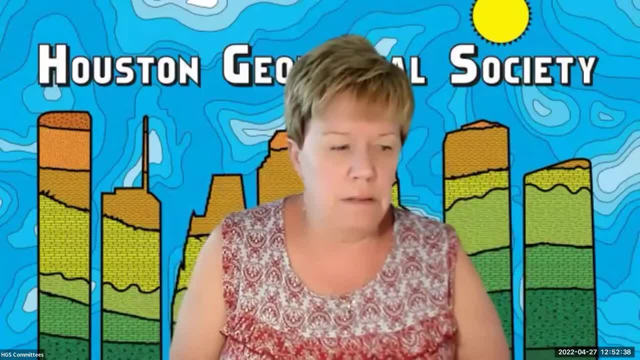 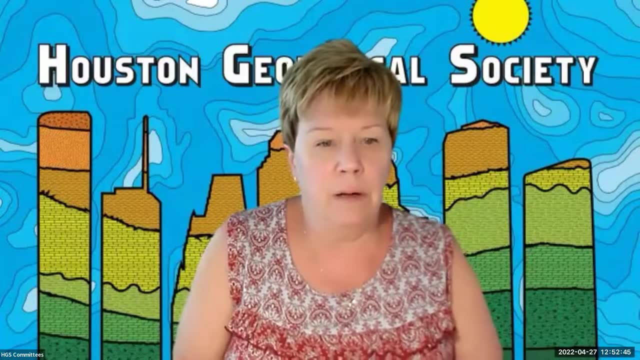 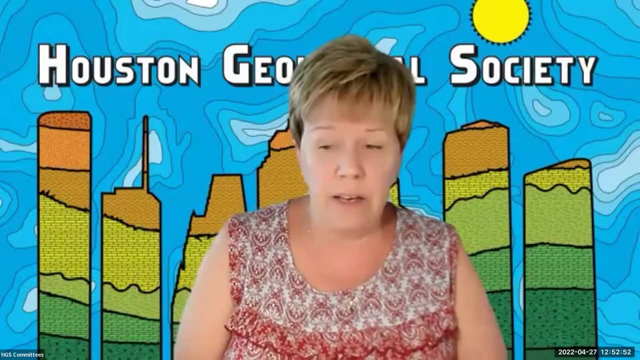 I mean we, we saw that work in Africa and Southeast Asia. They are huge in going into these areas And you're right, they have a different economic metric Then most you know international oil companies have. So they can go in at times and shoot seismic and pay money for stuff. 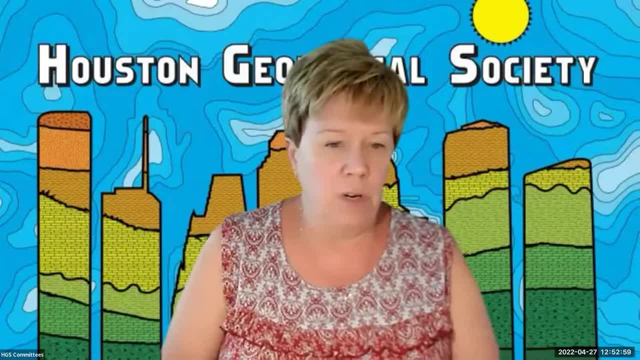 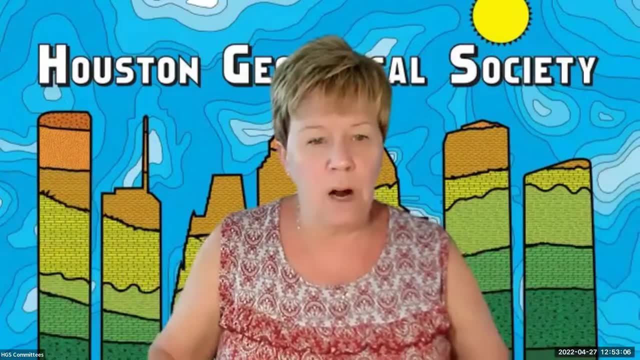 that would never make an economic hurdle in other companies. So it's, it's challenging. So it is. you know as much as we talk about in geology. you know we follow the rocks. We do as scientists, But as an explorer, you're still in here to make money. 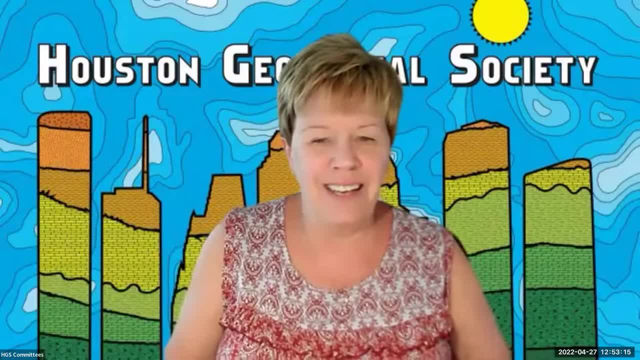 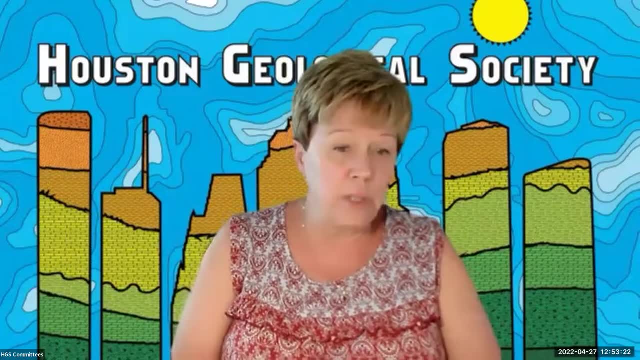 None of us are in here to lose money. It's a real fast way to go out of business, And so you do have to understand this, all of this commercial side and the engineering and what it takes to bring these, these resources, to bear. 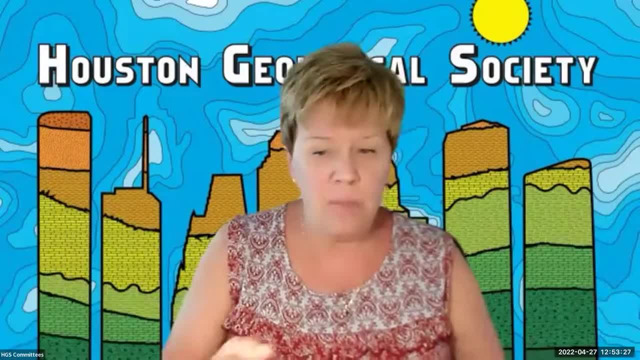 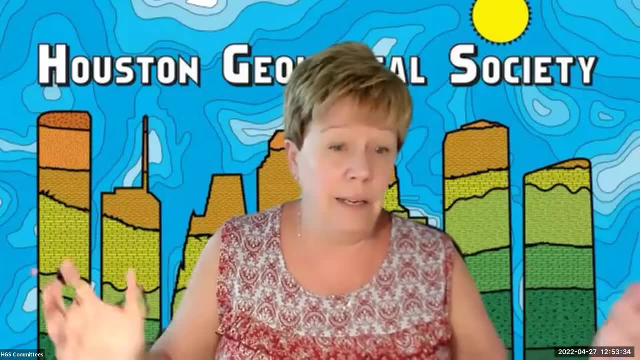 So you start with fundamentals, right. Where are the good rocks? And Michael, we used to call those countries, we called those basins arrested. So they had either a political overlay, You know, I mean Diana was in force majeure. 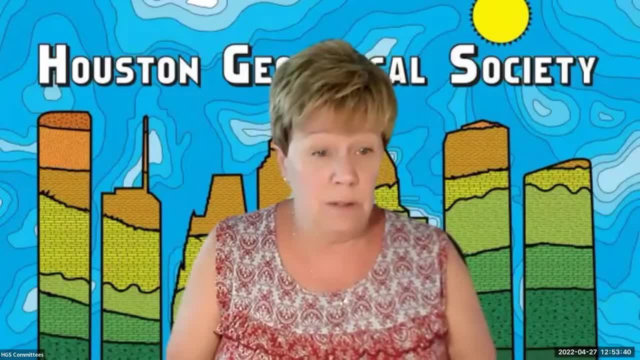 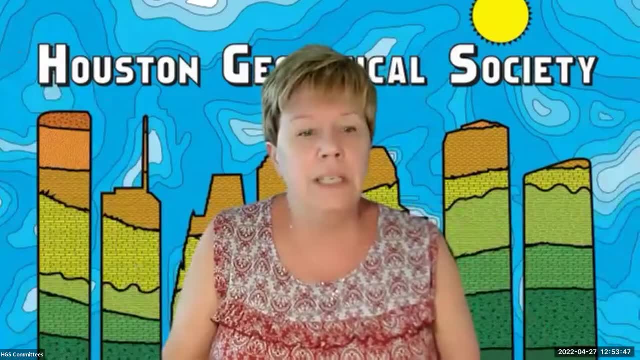 with both Suriname and Venezuela for 12 years. That's why nothing happened. So you know. and now it's like, oh, how did everybody miss this? People didn't miss it. You just couldn't do anything right Politically, financially, you really couldn't do much of anything because of that. 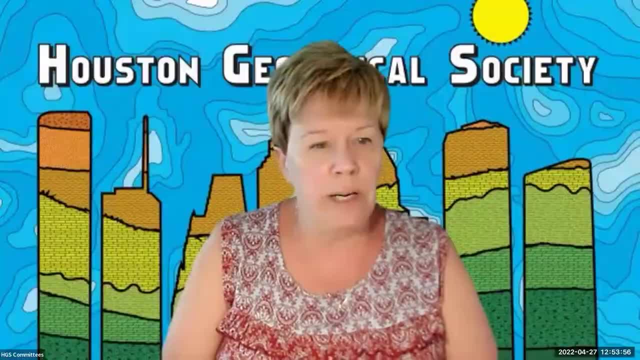 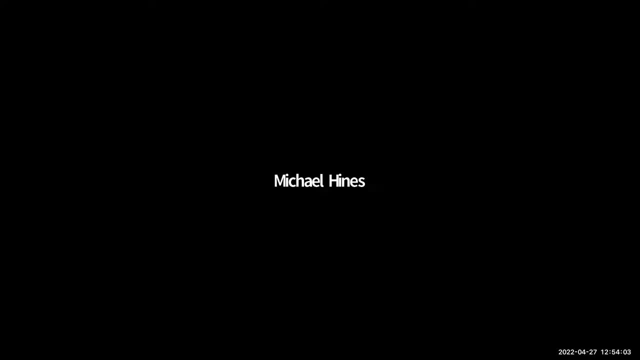 You had to wait for that to play out. It's hard to wait. Yeah, it's interesting. Even in Guiana, the northern part of the Cerberus block is still in dispute. Yeah, it is probably huge potential there, But it's in dispute with the Venezuelans. 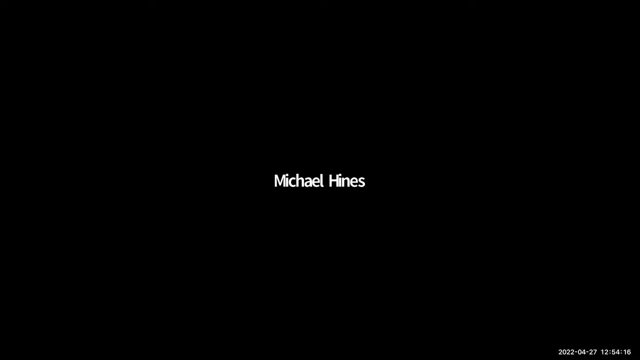 And of course we're biased that we have Guiana. That's it Because Venezuela has done quite such a great job with the massive amount of resources they already have that they clearly need more. Yeah, Whereas the Guianese, I would say on. 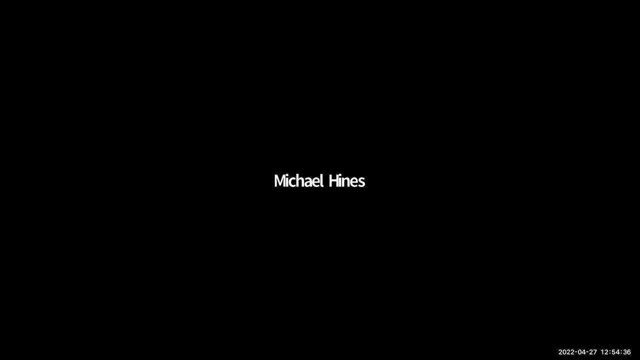 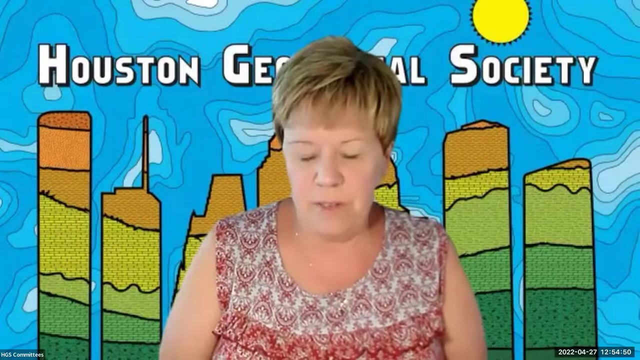 the two countries I think in the world it's Guiana and Norway that have done a very good part on their resource management. They're probably the best I've ever seen and worked in many countries. Yeah, I was telling David, I think Guiana, they actually have folks from the Norwegian. 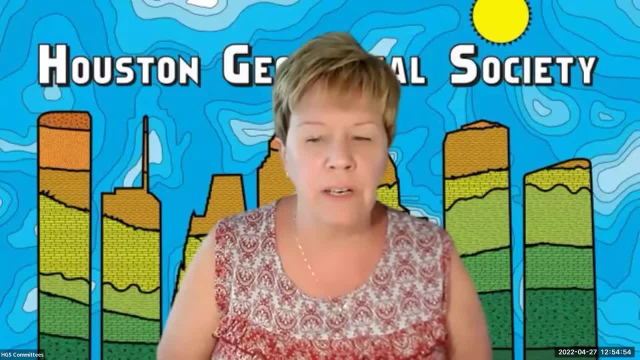 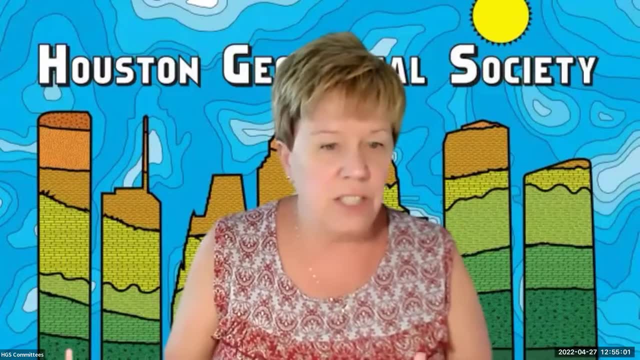 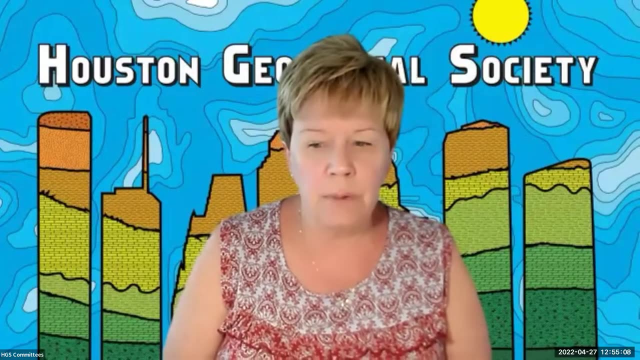 Petroleum Directorate that have been on their advisory boards early on, And I think that's a super smart move, because you really hate to see them go the way of Nigeria, which would be- And Angola to some degree. I think Angola did a better job than Nigeria, but still a lot of corruption. 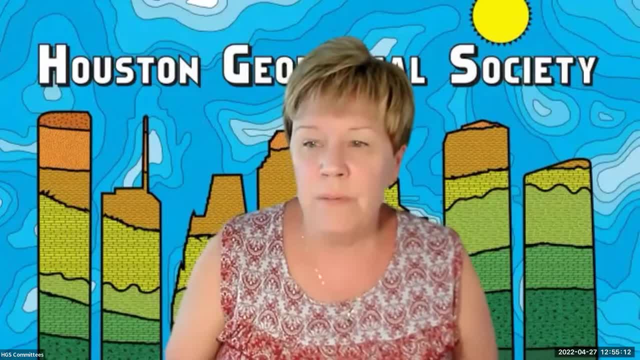 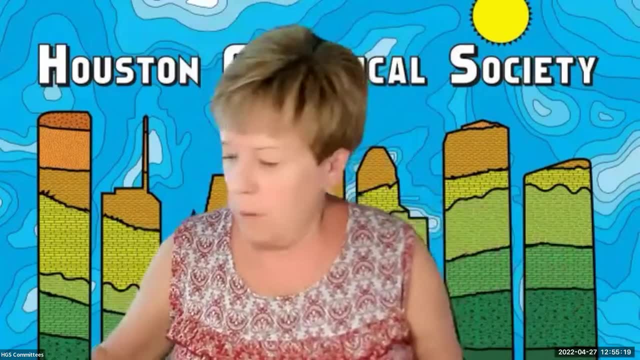 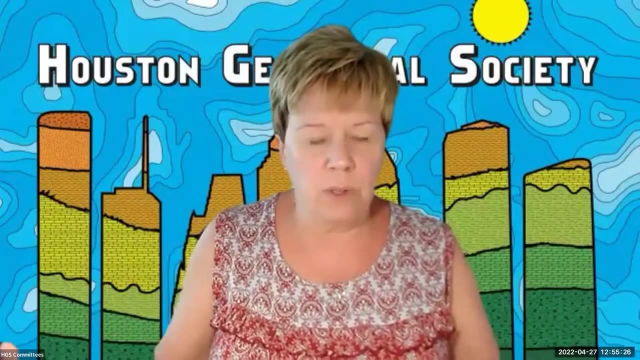 So cool, Okay, Do we have. So do we have other questions? We're coming up. We're coming up basically on our time. I appreciate the conversation. I personally find this fascinating because we talk a lot about all this resource that's. 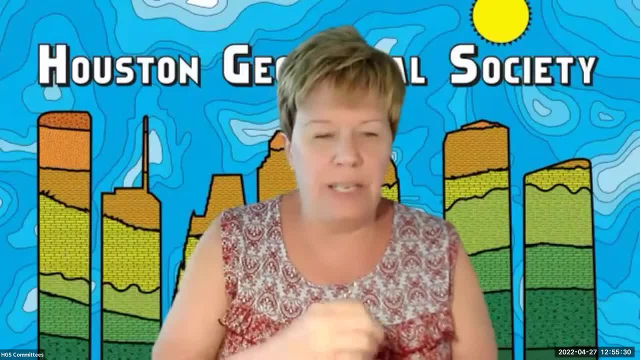 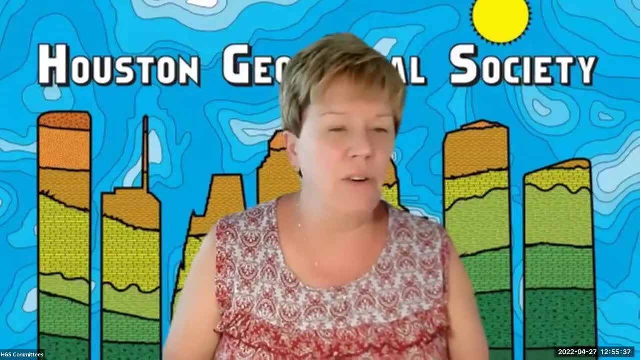 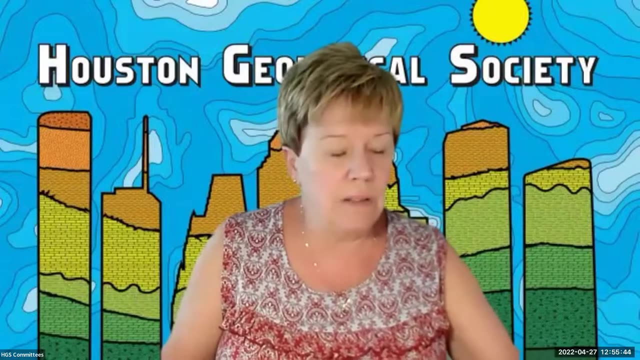 come on, that's been discovered, but until you can actually get it to market, you know it's basically, you know it's energy sitting in the ground And I worry that as we go through the energy transition, there will be less and less. 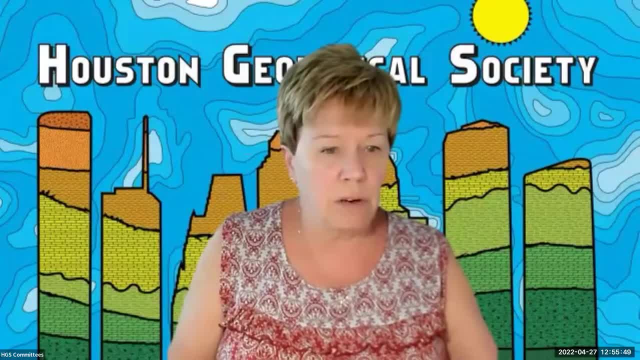 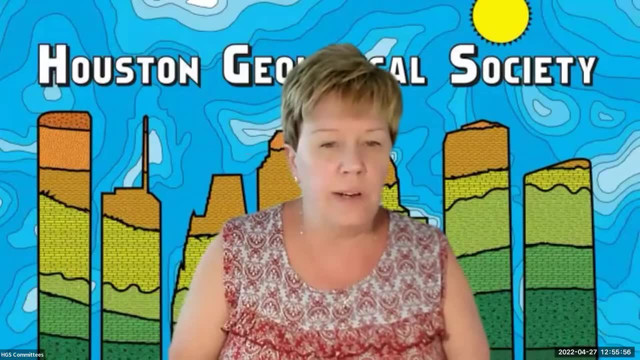 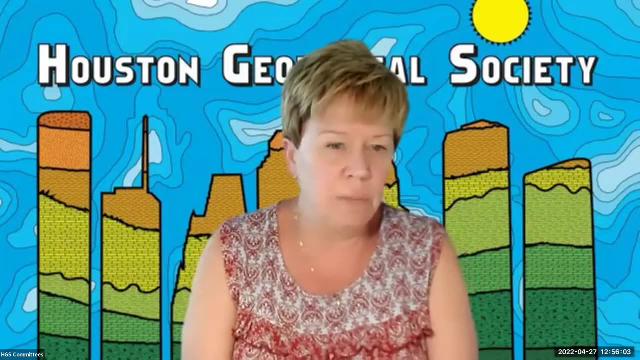 incentive to get some of this resource out of the ground. Now, if you're a third world country or you're even not one of the OECD countries, you're going to want to utilize whatever resource. you've got Many of these areas. it was interesting in your GDP chart and your NPV chart that country. 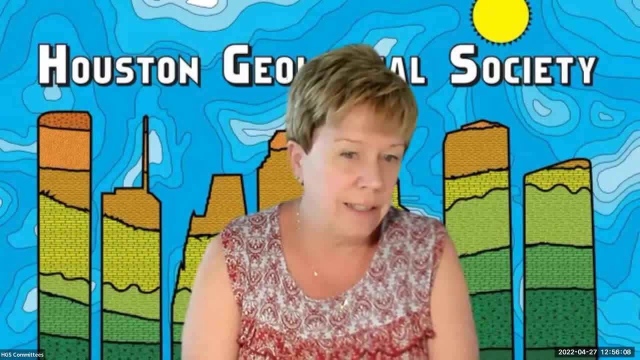 though, has to have the economic wherewithal to bring it online- I think you had said that- or they've got to be able to get a partner that's willing to come in and do it. So without some of this, Yeah, 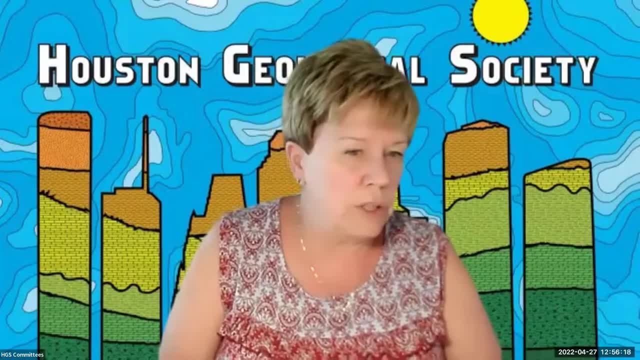 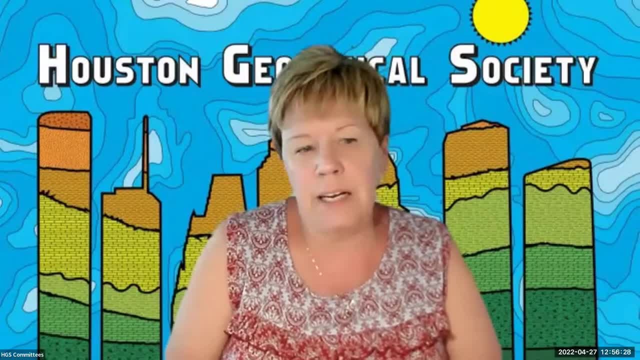 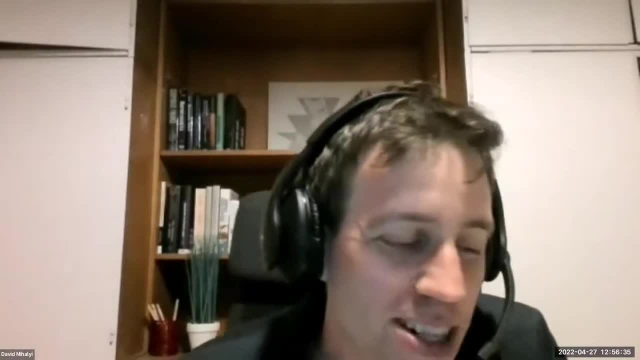 David especially. I mean you're at the World Bank. A lot of people come to the World Bank for financing. Yeah Well, the World Bank. I won't comment on the bank, But like yes, I mean countries are. many countries that I worked in are waking up that. 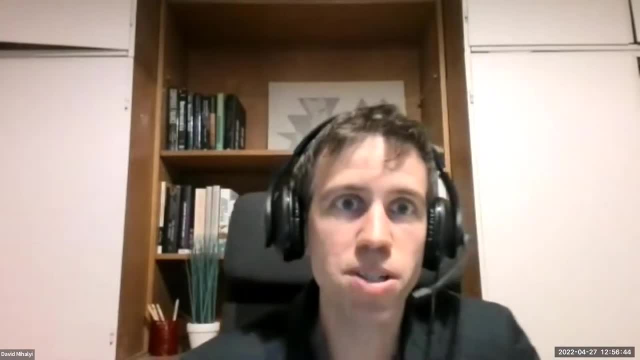 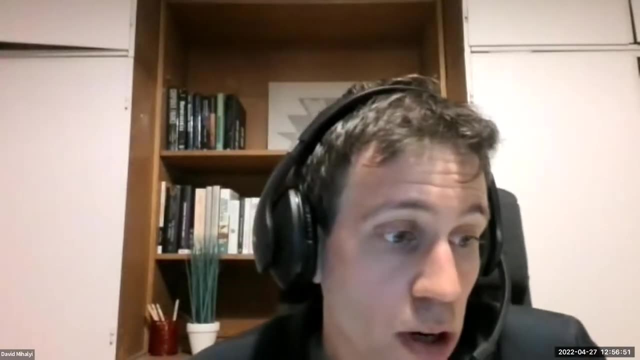 you know whether there's? you know how many super cycles like this are we gonna have anymore? is it the last one? um, so yes, there is definitely that kind of wake-up call in in places. i think the senegalese government was the one that put out statements. 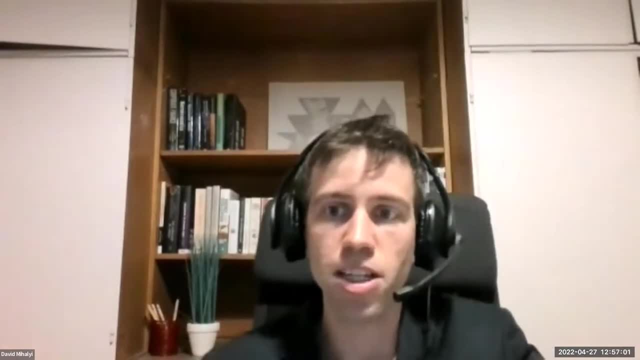 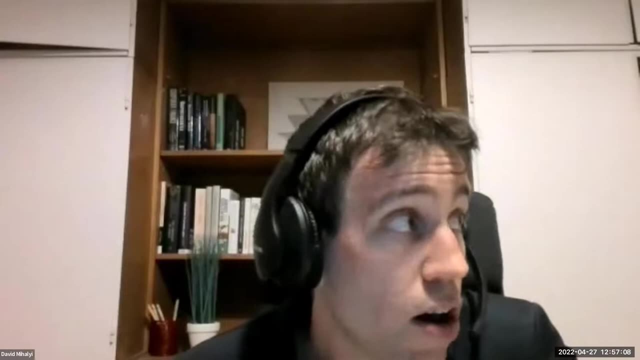 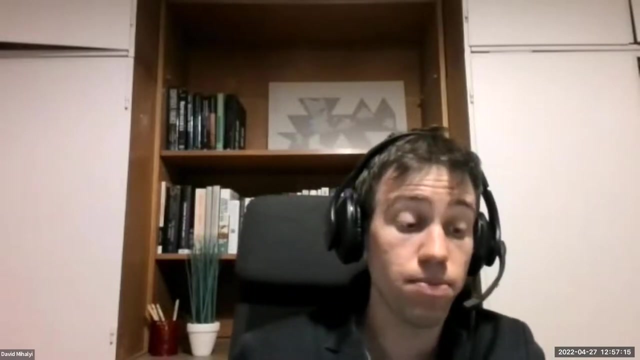 of this, so not no long ago, saying, you know, they see this this big last chance and they maximize on that. yeah, so, uh, so i think that's that's definitely uh, high, high on, on, on on their mind, uh and um, and also obviously the idea. the other part of the element is their own domestic. 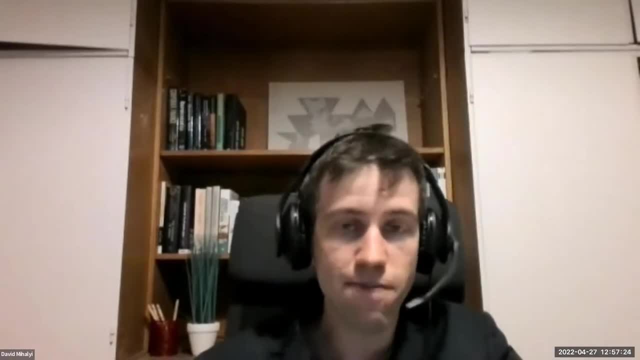 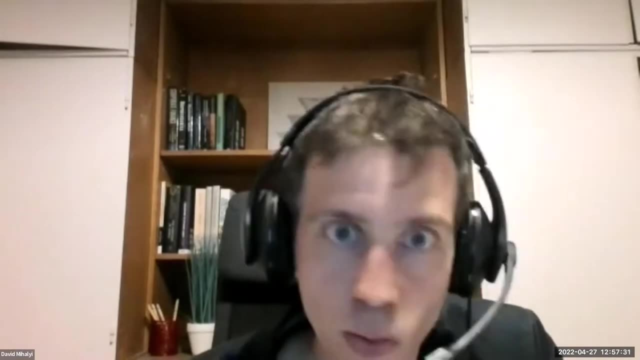 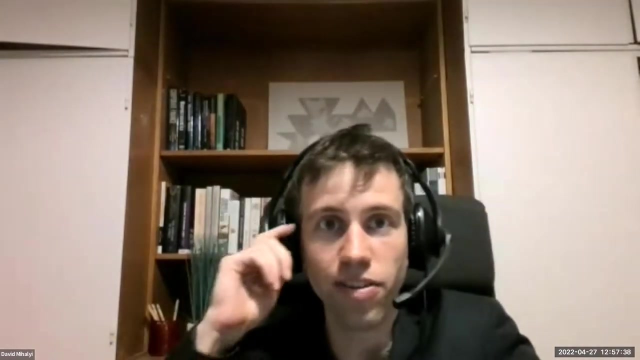 energy needs, right, i mean, these countries, um, have have been barely using any and so they also might be skeptical to look at. uh, you know, say, the west, uh, rapidly decarbonizing, which is great and needs to happen, but they, you know that that doesn't mean that they want to completely. 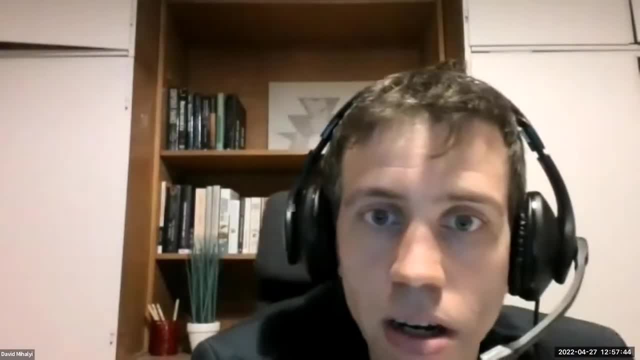 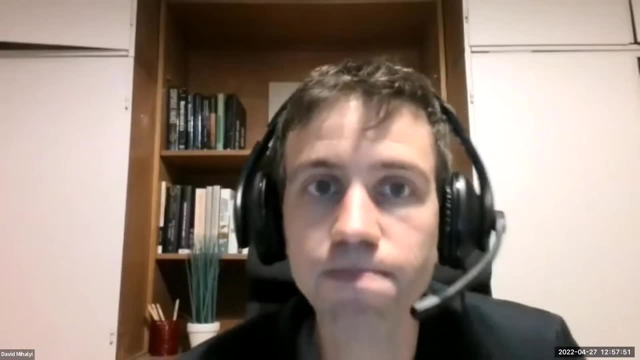 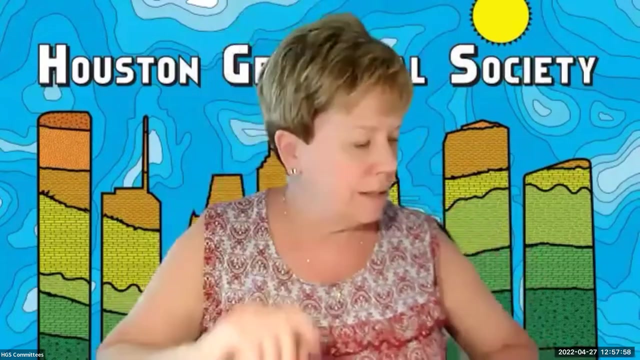 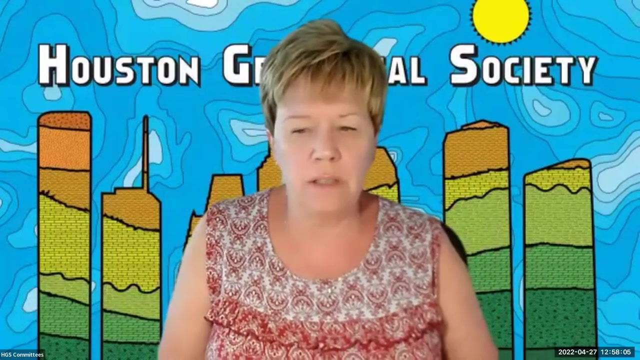 i mean, they don't see how they could, you know, skip um developing, you know, their own resources and their own energy grids, and all that all right. well, i want to thank david for giving what was a fascinating talk and again, this will be available um on the hgs youtube site, where we store our 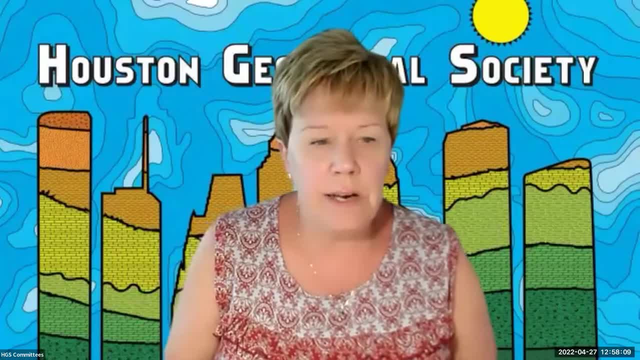 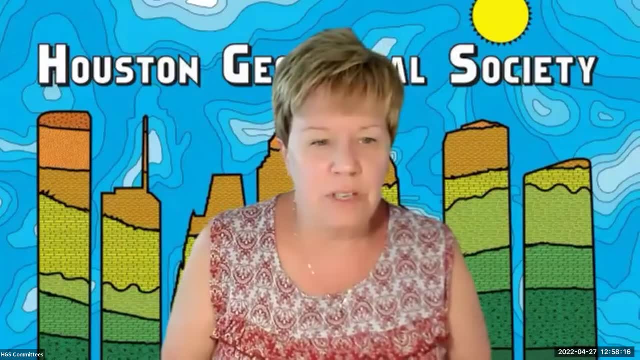 technical talks. and again, if you have any follow-up questions for david um, his contact info actually is on the hgs youtube site and i'll see you next time. bye, at the hgs website as well. go look at the seismic. i think that'd be an interesting follow-up to your. 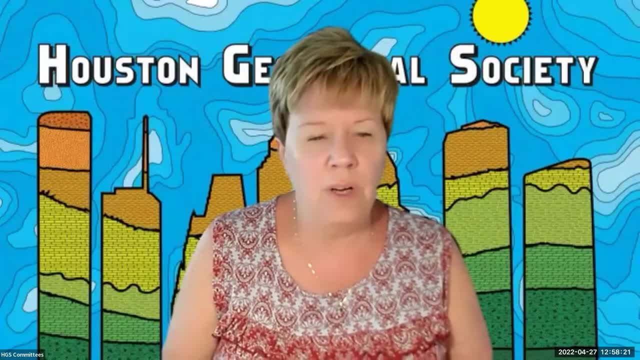 your wells drill data set as well. so thank you very much, appreciate this, and i am going.